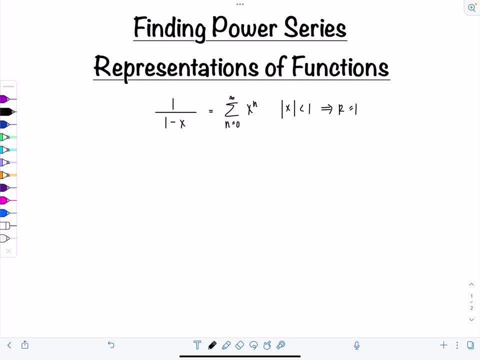 depending on what the function looks like, you're going to do one of three things. If it resembles this enough- but maybe this term is a little bit different- there's some extra stuff going on in the numerator. all you're going to have to do is multiply, divide, add. 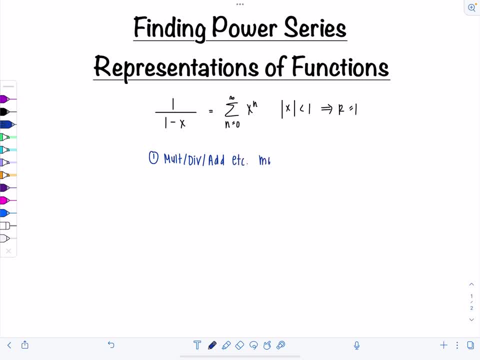 etc. Do some clever things To manipulate the original sum. n equals 0 to infinity, x to the n, And you're done. The second case is if you have 1 over 1 minus x to some higher power down here, I don't. 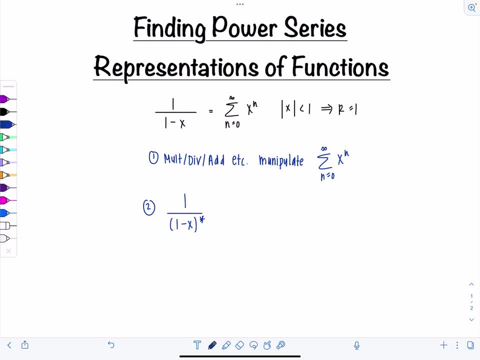 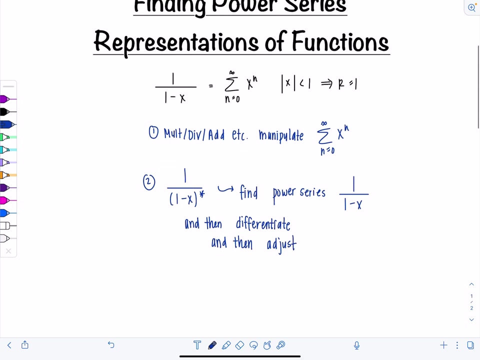 usually start busting out the binomial series. What I do is find a power series To please sound easy. I don't're going to do that for the moment. I'm just going to add Retroarmed, and then what will happen here is, if I break that, it's not going to kind of change And then I'm going. to increase the value of 2 over 1 minus x. This is a lawyer skilfully out of keep away concept. So that said, if I have 1 over 1 minus x, I'm going to Danielle too, and I'm also. 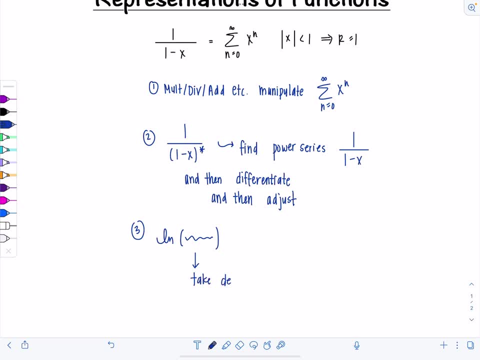 going to work the equation. so I'm just going to have topel applied okay To, To some version of 1 over 1 minus x or whatever it may be, and then you differentiate and then adjust. gonna do is take the derivative, find a power series for the derivative and then 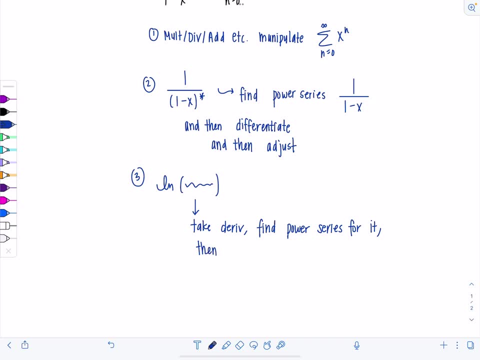 anti-differentiate that to undo it, integrate it and adjust. You'll see what I mean. You'll see what I mean as we start working through. but there's really only three cases. So I think when you remind yourself of that, it will feel. 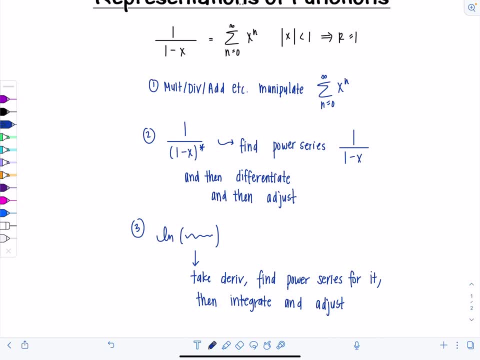 less overwhelming, okay, And we're just going to jump right in and do some examples. So if you're one of my students, I'm going to start off doing some easier stuff from the homework, just to kind of like refresh your memory, and then we're. 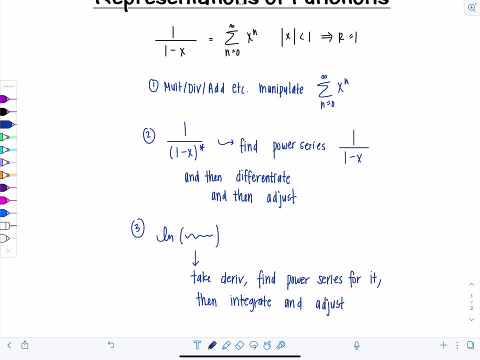 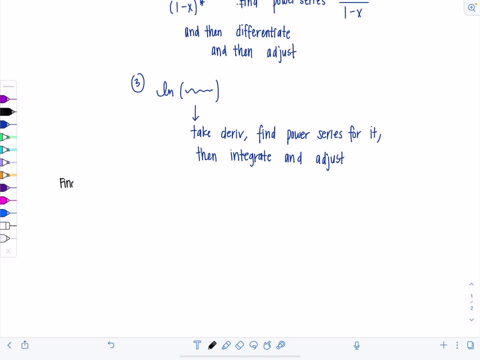 going to work on the last few spicy ones from the practice test. okay, Here we go. So the directions are basically: find a power series representation, And then sometimes you'll keep in mind that the original answer to the formula is always mod 1 plus the power cut-off of writing it, And we're going to completely. 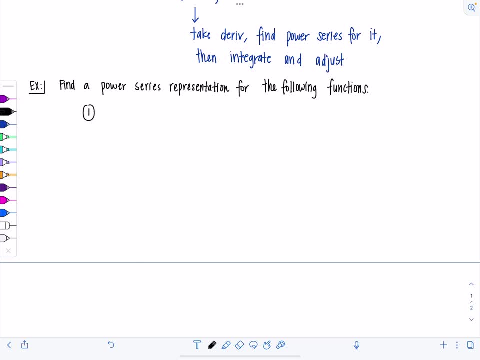 modify the formula now. so very quickly, okay, just like that, just to explain and then to continue, and then let's get going, Let's go on, Let's go on. All right, what did I tell you home base was? 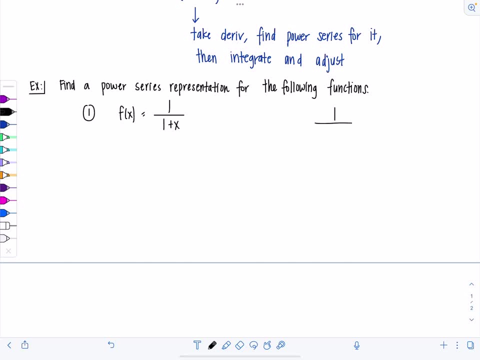 You've got to memorize this: 1 over 1 minus x is the sum. n equals 0 to infinity, x to the n, And the radius of convergence is 1.. How can I make this f of x resemble that home base? 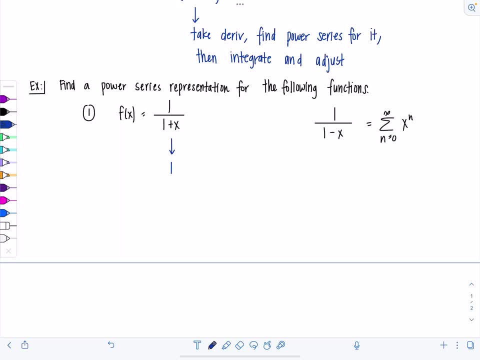 Oh well, it's not too bad. I already have a 1 in the top. I love that there's a 1 here. I just wish that plus x was a minus x. So I'm going to make it happen. I'm going to write it as minus negative x. 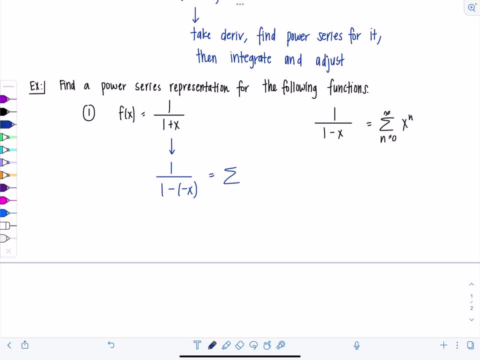 And then how does that affect what I'm writing in my infinite series? Well, now I have the sum n equals 0 to infinity, And instead of x to the n, I'm going to have negative x to the n. Do you see that? 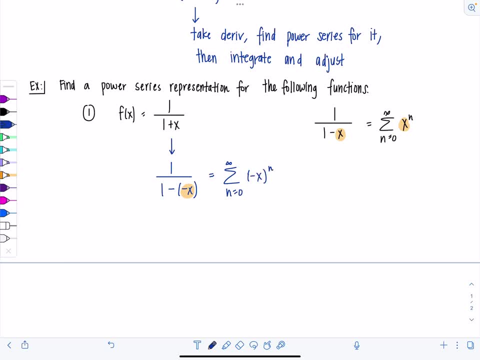 Oh good, And then no, you don't leave your final answer like that. You're going to split up the negative from the negative, x to the n. So we write this as: n equals 0 to infinity, negative, 1 to the n, x to the n. 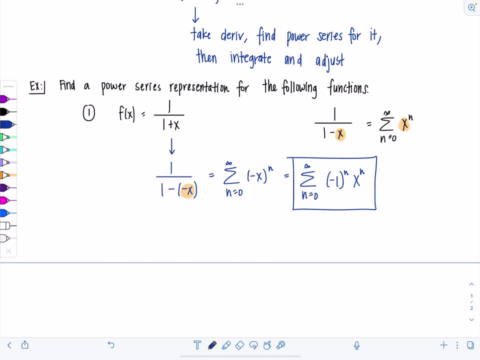 You want to try to leave it, so it's just x to the n at the end whenever possible. If we're going to find the radius of convergence, easiest thing to do is go to the step right where you first wrote your sum, because this is r right. if we're thinking of a geometric 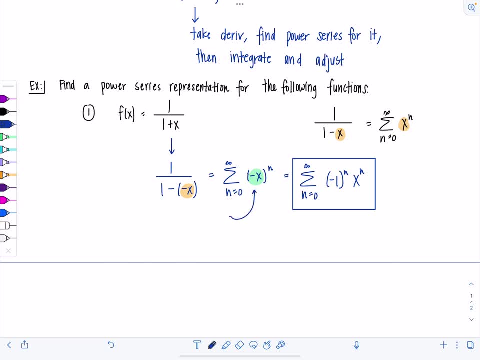 series And we require at this step- if you think back when you first learned geometric series- we require the absolute value of r, in this case, absolute value of negative x, which is just absolute value of x to be less than 1.. 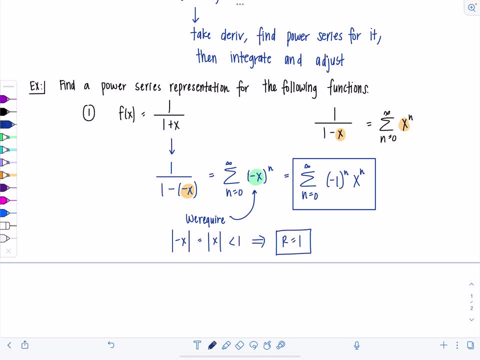 So that means the radius of convergence is just 1.. And the interval of convergence- if anyone were to ask- is from negative 1 to 1, not including the endpoints. How do I know that? I didn't even do a ratio test or anything? 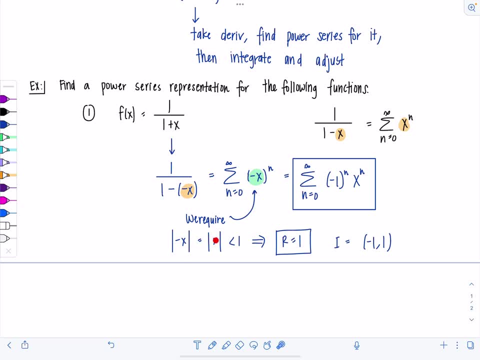 I don't need to Because, remember, geometric series diverges if r is equal to 1 or negative 1.. So I know for sure that these endpoints- 1 and negative 1, will not be included on the interval of convergence. 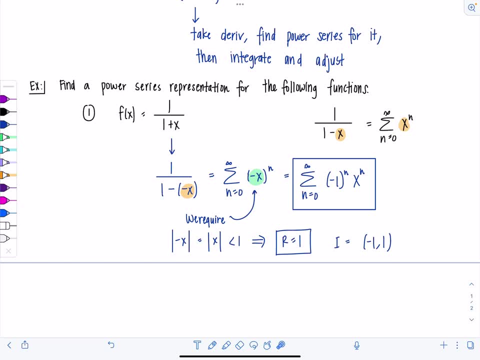 I don't need to spend any more time thinking about it. This is only true for power series like this. okay, All right. good, That was not so bad. That was a warm-up, Let's do another warm-up. Example 2, f of x is 2.. 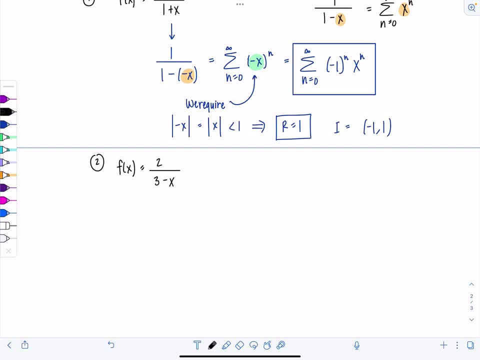 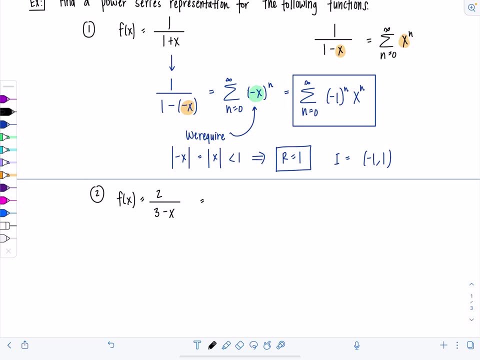 2 over 3 minus x. Oh, oh, oh, oh. So this looks rather different than 1 over 1 minus x, but we can adjust. I can write this as 2 times 1 over 3 minus x, right. 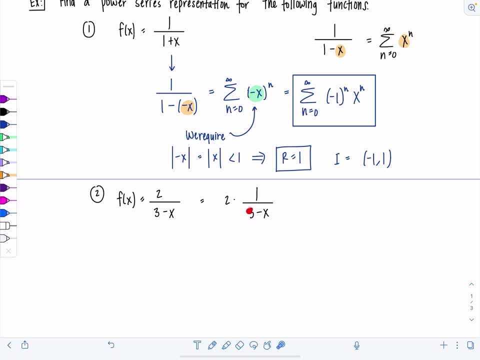 But then you know, I'm still not happy. I need a 1.. This is a 3.. How do I adjust? I divide out or I factor out that 3 from the denominator, So this is 2 times 1 over. 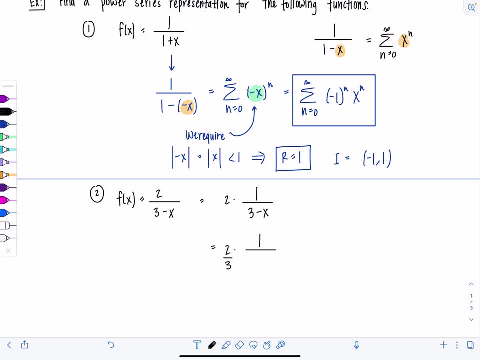 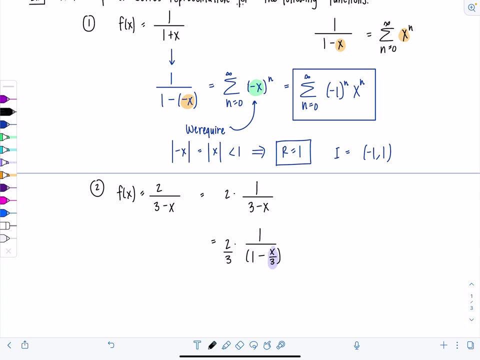 Let me take the 3 out here. Nobody have a panic attack. And then this is 1 minus x over 3.. Ooh, okay, Are we all right? Good, So basically this is my r now, okay, And I just have an extra 2 thirds hanging out front. 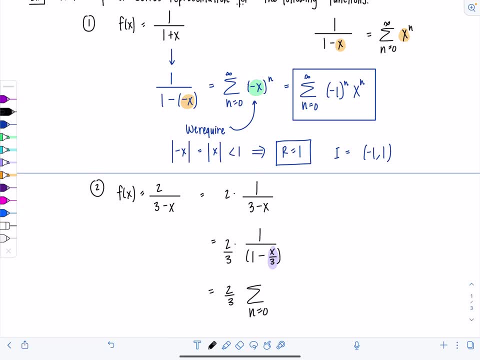 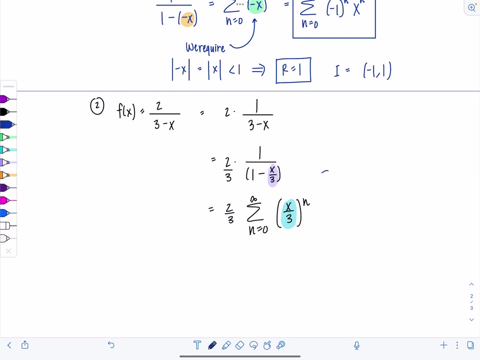 So I have 2 thirds times the sum. n equals 0 to infinity x over 3 raised to the n: Boom. If you want to find the radius of convergence now go for it, Or just remember this is the step to come back to, right here. 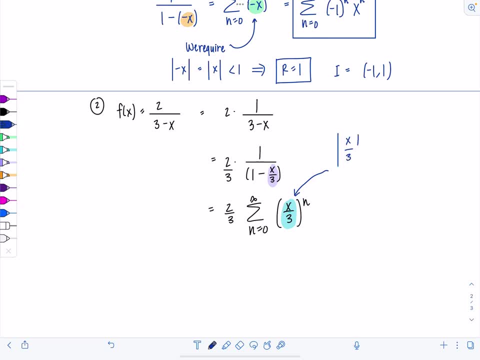 Because we require absolute value of r to be less than 1, which means absolute value of x has to be less than 3.. So my radius of convergence is 3.. Interval is from negative 3 to 3.. Okay, I mean, that's done. 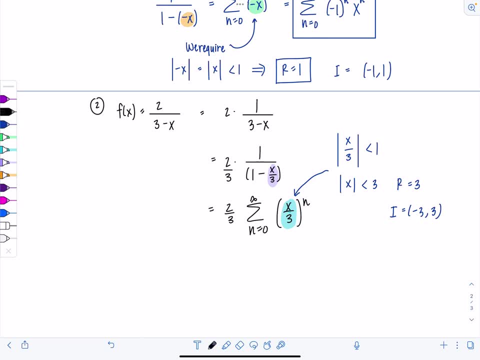 So let's clean this up, Let's clean up the series now. So you want to try to leave it as x to the n in the final step. So we have 2 thirds: sum n equals 0 to infinity, x to the n, over 3 to the n. 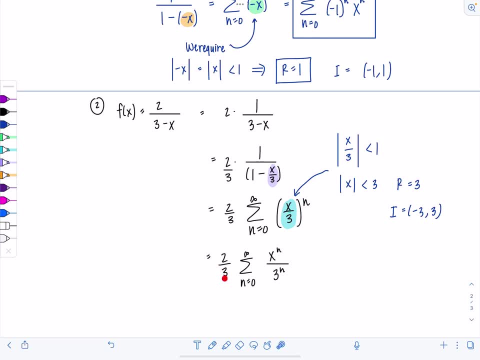 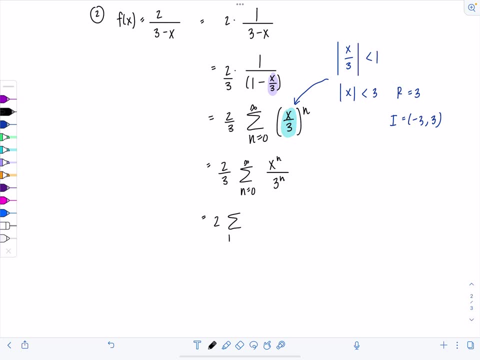 And then it will be useful. Let's see how. there's a 3 out here. Bring it inside the sum. I'm going to leave the 2 out, though He has nobody to join with inside the sum, So just leave them out. 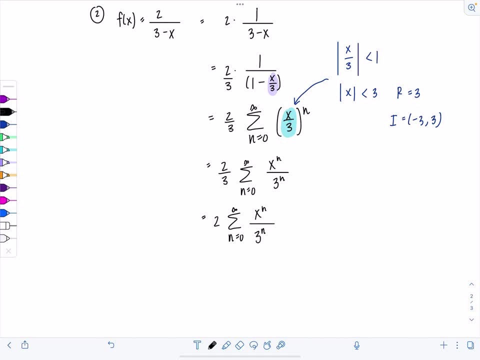 They're like a little loner. Okay, x to the n over, 3 to the n plus 1.. That's it Good. So we're still doing the first case where all it just takes is some, you know, manipulation using arithmetic. 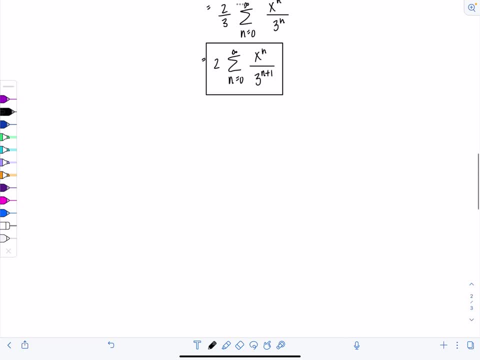 Arithmetic. that's all we're doing. Okay, let's try another before I start upping the spice level. Okay, f of x is x squared over x to the 4th Plus 16.. So how are you going to make this resemble 1 over 1 minus x? 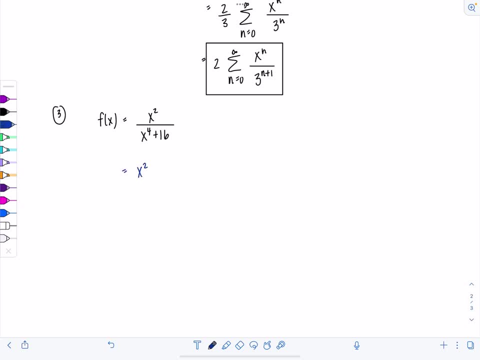 First things first. I'm moving that x squared away right, And then I have times 1 over. Why don't we write this as 16 plus x to the 4th? It makes me feel better when the constant's first. 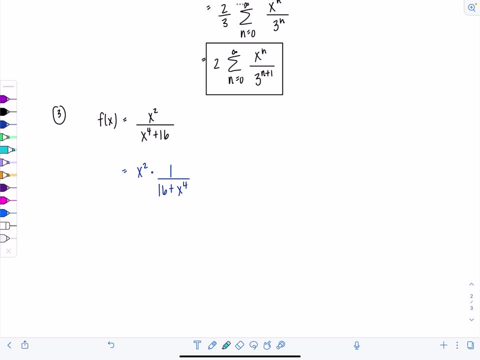 Doesn't it make you feel better? Other issue is: I need this to be a 1.. So, again like last time, let's factor out the 16. And then I have 1 over 1, plus x to the 4th over 16.. 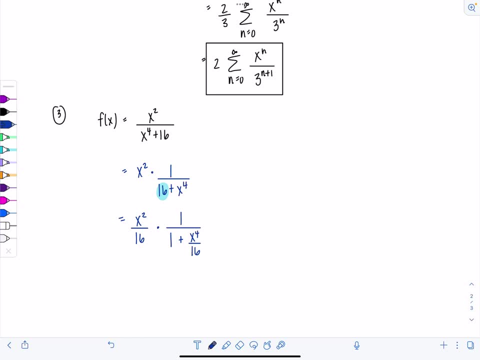 Is this good? Can I write a power series? Not yet Make that subtraction. So we have x squared over 16 times 1 over 1, minus negative x to the 4th Over 16.. Beautiful, Okay, So focus right here. 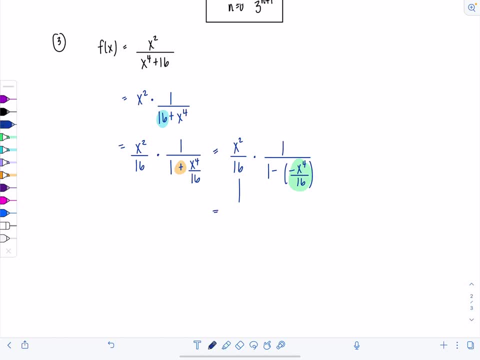 This is your r, And then this stuff just hangs out: Okay, x squared over 16.. We'll deal with it later. Sum n equals 0 to infinity, negative, x to the 4th over 16 to the n. Okay. 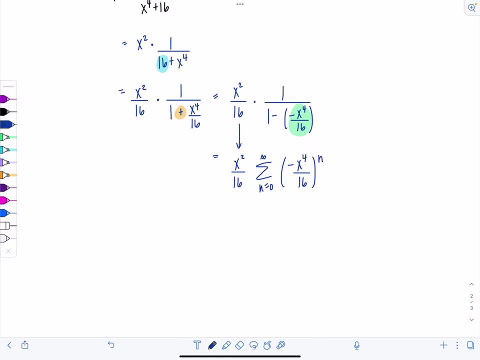 Let's see. Do you want to find the radius of convergence now? Why not? Here's r. We know that this sum converges if the absolute value of r is less than 1, which would mean the absolute value of x to the 4th is less than 16.. 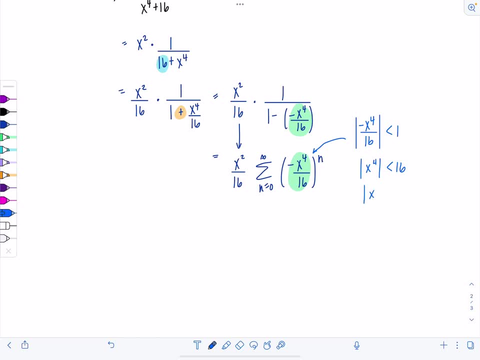 And that happens if absolute value of x is less than 2.. So radius of convergence is 2.. And the intervals from x to the 4th is less than 2.. And the intervals from negative 2 to 2.. All right, 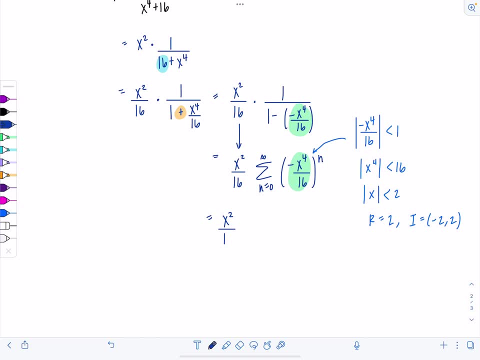 Now let's clean up. So x squared over 16.. Sum n equals 0 to infinity. Now distribute the power of n to this negative, to x to the 4th and to 16.. So you're going to have negative 1 to the n, x to the 4n. 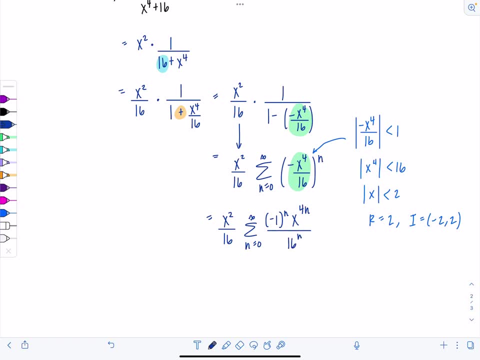 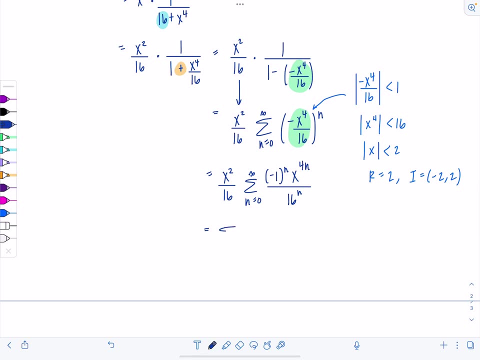 Over 16 to the n. Okay, And then let's go ahead and bring in what's on the outside. So we have: sum n equals 0 to infinity, negative, 1 to the n, x to the 4n plus 2.. 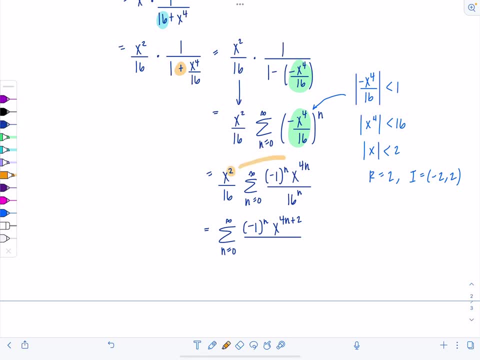 Why 4n plus 2?? Because I'm bringing x squared inside the sum now. So if you have x to the 4n times, x squared, That's 4n. That's x to the 4n plus 2.. 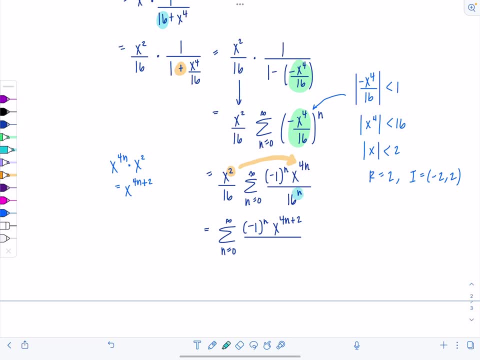 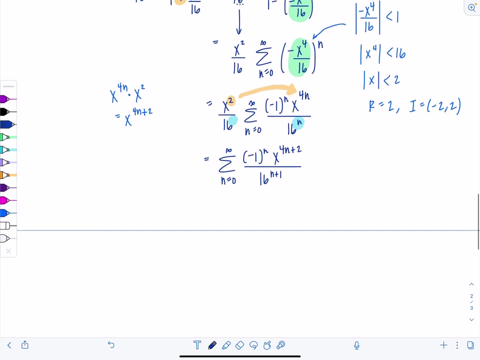 Okay, And then similarly down here, you see I have 16 to the n and then I have one more, So then that would be 16 to the n plus 1.. Now you could stop here, but technically, like 16, we can break it down as 2 to the 4th raised. 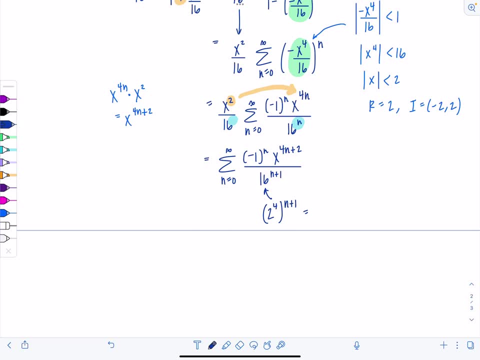 to the n plus 1.. And then that would be Remember, This would distribute 2 to the 4n plus 2.. And the reason that's just a wee bit more desirable is because, well, 2 also matches the radius of convergence. 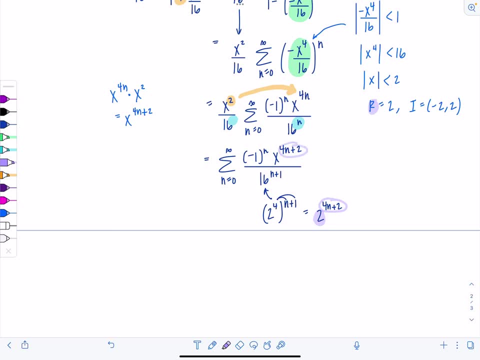 And then notice this exponent is the same one that I have on x, So that is a more desirable way of writing it, guys. Yeah, I know. So we have the sum n equals 0 to infinity negative, 1 to the n, x to the 4n plus 2.. 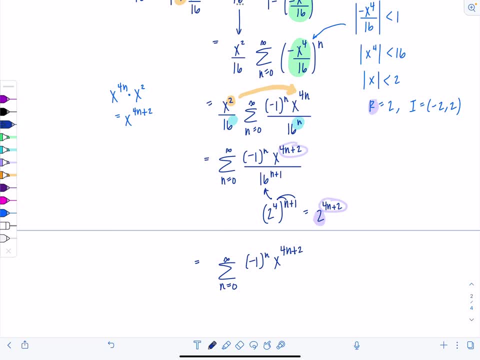 Okay, Okay. So we have x to the 4n plus 2 over 2 to the 4n plus 2.. Yes, Box that one with pride. Job well done, Job well done. Okay, Let's up the intensity just a wee bit now. 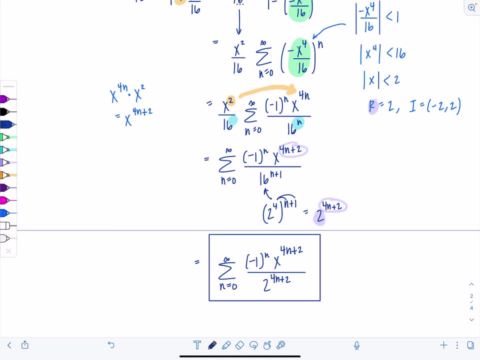 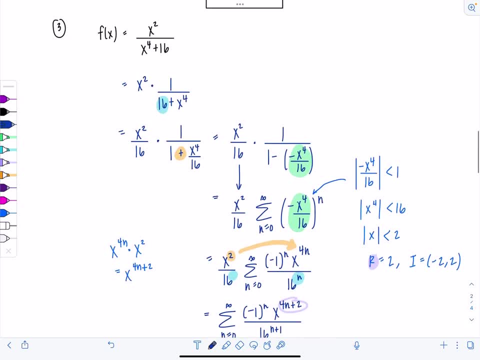 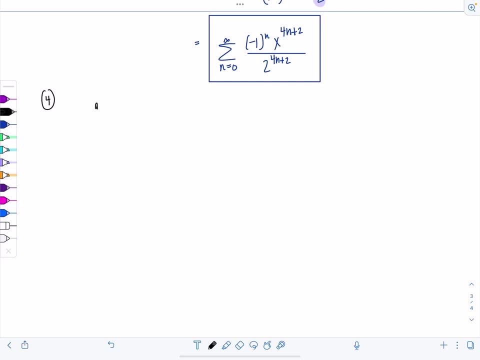 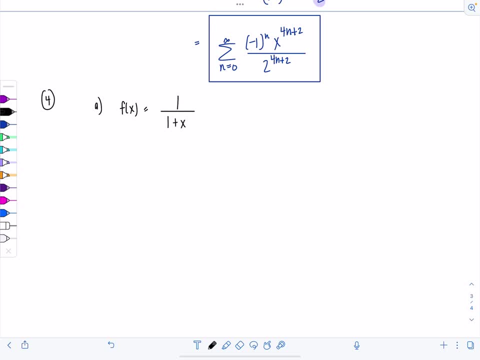 This is going to be a little different, for a F of x is 1 over 1 plus x squared. Ooh, This is the second scenario. now, Okay, Anytime you see an exponent down here, what you're going to need to do is first find a. 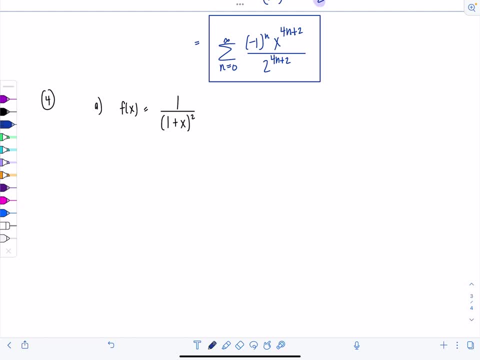 power series for the plane version Plane. enough for the plane Plane version being just 1 over 1 plus x. Then you're going to differentiate the appropriate number of times to make that exponent. I'm going to tell you something right now that I learned the hard way. 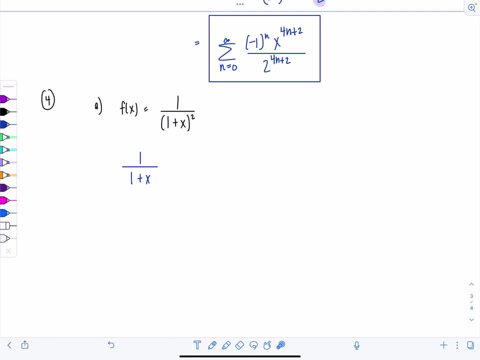 You don't want to square an infinite series? okay, So don't say, oh, I'm going to find the representation of 1 over 1 plus x and then just square it. That sounds great, I know it sounds great, but it doesn't work out. well, okay, Don't square an infinite series. I always wanted to. 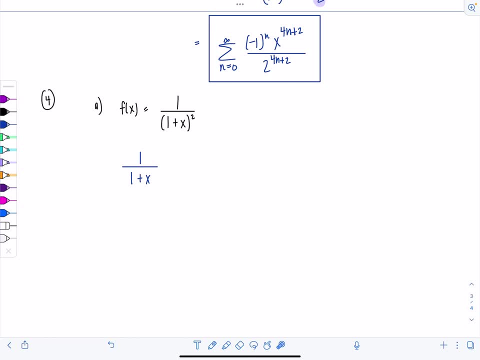 It never was the answer and I'll tell you, if you're in Calculus 2, you're not going to need to. I'm not saying you're never going to need to in your entire math career, but it won't be necessary. 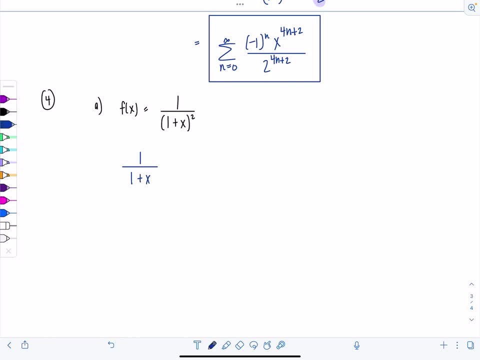 in this class Got it Great. Okay, so 1 over 1 plus x. we did that one already at the beginning of the video. Think of it as whoa: 1 over 1 minus negative x, right, Right. So then this is the sum. 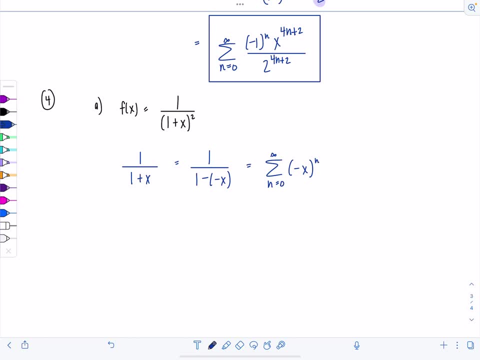 n equals 0.. 0 to infinity negative x to the n, which is the sum. n equals 0 to infinity negative, 1 to the n, x to the n, And we know radius of convergence for this guy is 1.. Great, So how am I going to? 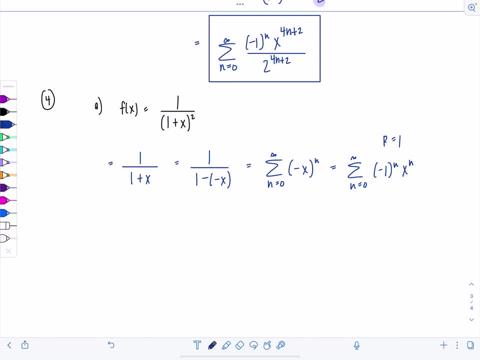 make it squared in the denominator. Well, I want you to remember that 1 over 1 plus x is 1 plus x to the negative loop first. yes, So what we're going to do is take a derivative Instead. okay, So the derivative with respect to x, of 1 plus x to the negative first. 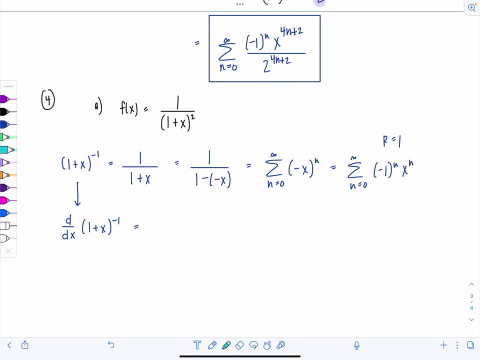 is going to be, let's see. so you take that exponent, bring it down in the front, so this is negative 1 plus x, and then subtract 1, my new exponent should be negative 2.. And then we do have to just think about the chain rule. You would multiply by the derivative of the. 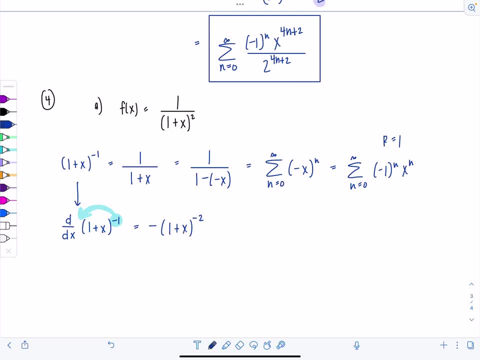 inside, but that's just 1.. Great, Now I'm going to take the derivative. because I took the derivative of one side of the equation, now I'm going to take the derivative of the other side. Don't be scared. Identify x. 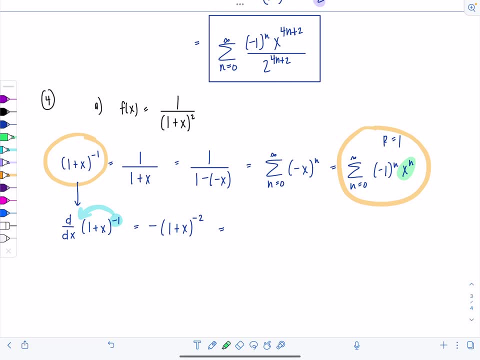 Where is x in the sum? It's just right here. Everything else is a constant, so don't mess with it. We're going to have the sum negative 1 to the n and then, if you take the derivative of x to the n, 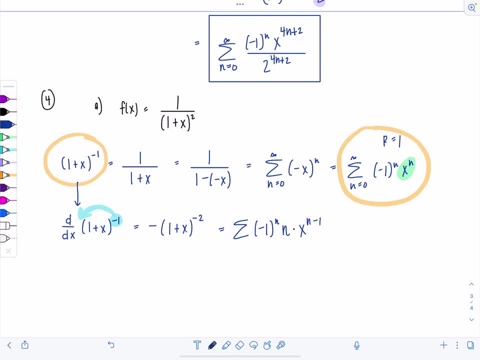 it's going to be n times x to the n minus 1.. You bring that exponent down in front and then subtract 1.. That's your new exponent. Now you have to be careful Anytime you take the derivative of an infinite series. check that index n starts at 0. If I plug in 0 for n here, 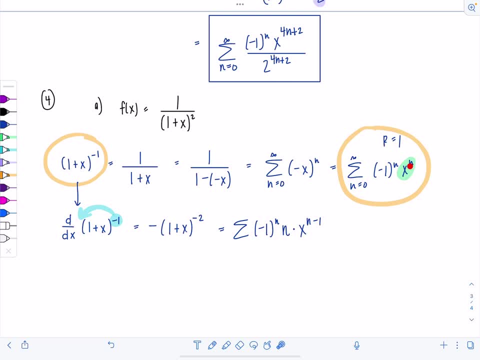 you're going to have negative 1 to the 0,, x to the 0,, which is just 1.. And that's a constant. So when I take the derivative of the n equals 0 term, it goes away. so my new sum is going to start at 1 to infinity. Let me write that out one more. 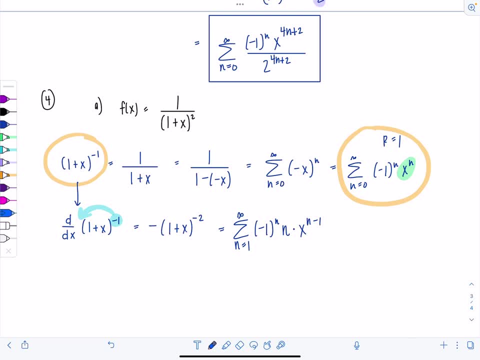 time because I feel like you probably are a little overwhelmed. I'm not writing out this whole sum, but the first term when n is 0 is 1, and then when n is 1, it's minus x and then plus x squared. 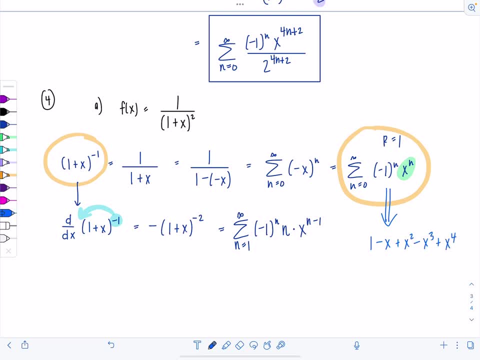 minus x, squared Plus x to the fourth, et cetera. right, This is n equals 0.. This is n equals 1.. And so if we take the derivative, well, this one's going to go away, right? So that's why the derivative starts at n equals 1.. 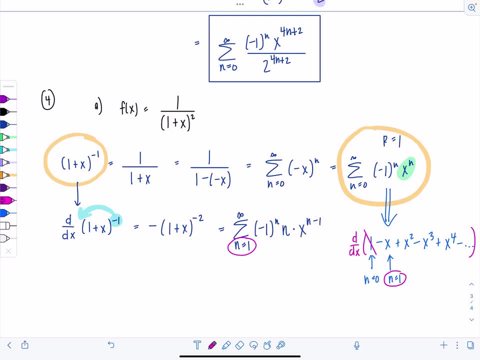 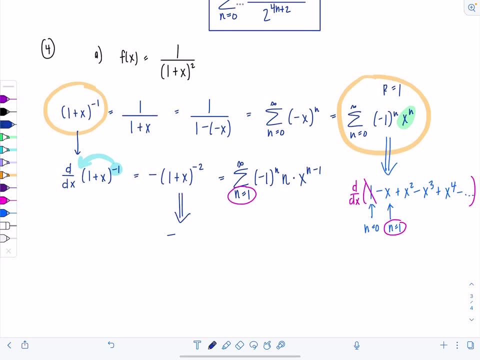 All right, Good. So let's see what have we done with ourselves. Are we in any better shape Right here? this is negative 1 over 1 plus x squared, That equals the sum n equals 1 to infinity. negative 1 to the n times n times x to the n minus 1.. 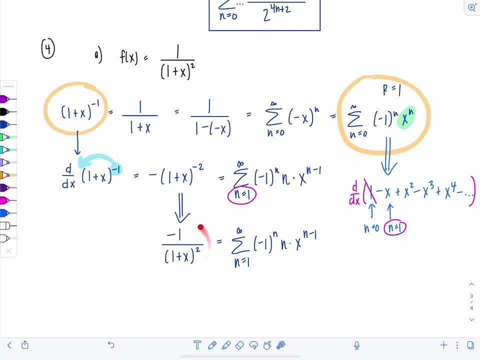 Is that what we want? Is that f of x? Let's look, Here's what I have. a power series for F of x looks super similar. It's just I got to get rid of this negative. Okay, So I'm just going to multiply both sides by another negative. 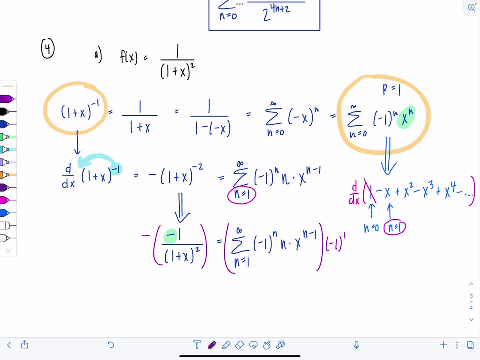 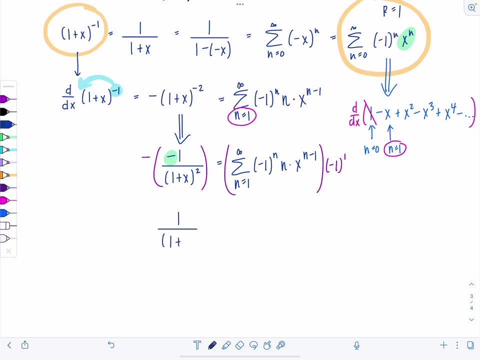 And that's the same as just multiplying by negative 1 to the first right. Why am I telling you that You're like I know? because I can combine that extra negative with negative 1 to the n. So now I have 1 over 1 plus x, squared equals the sum. n equals 1 to infinity. 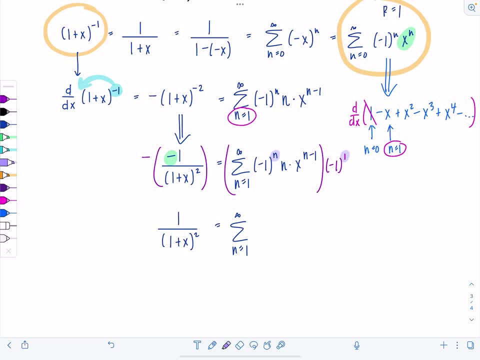 See how these two are going to combine. I have negative 1 to the n and negative 1 to the first, So that's negative 1 to the n plus 1 times n times x to the n minus 1.. All right, And then you do want to try to have your final answer with x just to the n. 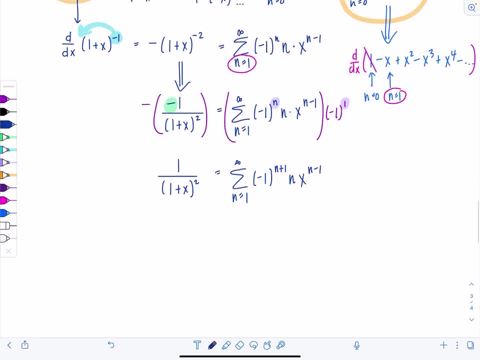 if possible. So let's see: If I want to make this n instead of n minus 1, I want that to go up by 1.. So if I want this, if I want this expression to go up by 1, I need to start the sum 1 lower. 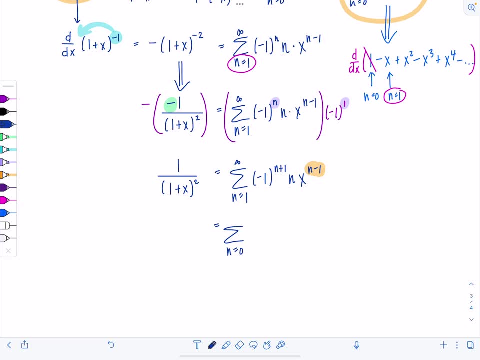 So I'm going to start at n equals 0 to infinity, And then now all of the n's become n plus 1's, So then I have n plus 1 plus 1, n plus 1, x to the n plus 1 minus 1.. Okay, So anytime you lower. 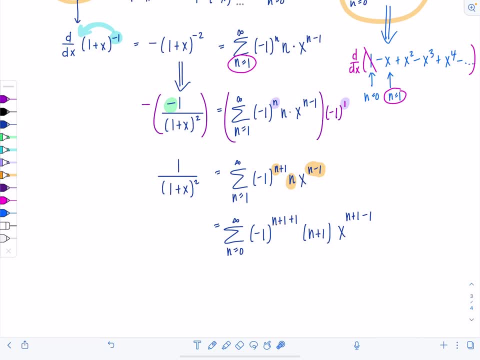 the index here you have to add To the expression in the sum by that amount. Now notice I have negative 1 to the n plus 2 over here, right Well, that's negative 1 to the n times negative 1 squared, which is just negative. 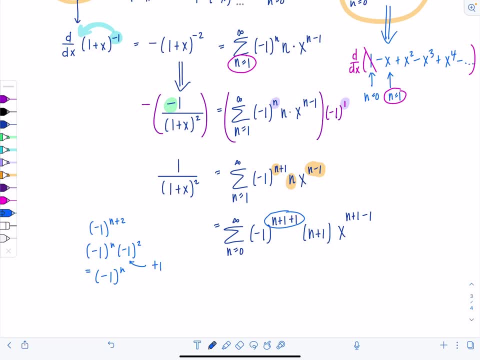 1 to the n, because that's positive 1.. So let's clean that bad boy up. So n equals 0 to infinity, negative 1 to the n, plus 1 times x to the n. Great, Now what's the radius of convergence for this series? 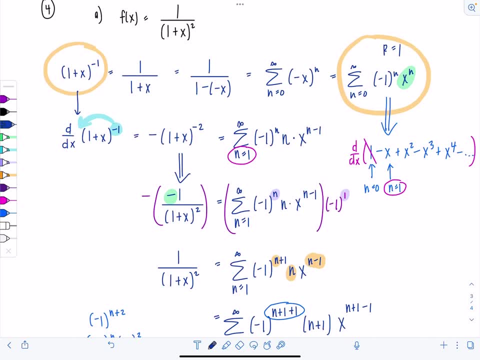 Well before we took the derivative, we knew the radius of convergence was 1.. And we have a fabulous theorem that tells us that the radius of convergence of a power series is preserved or it stays the same when you differentiate or integrate. So thank you, theorem. I don't need to check a single thing. 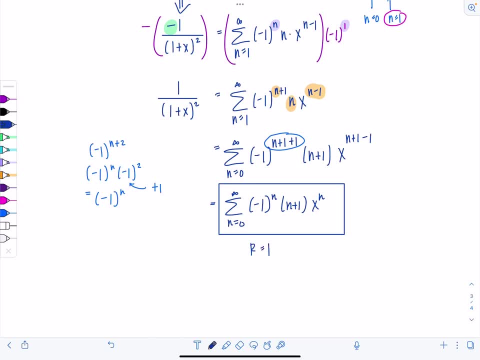 The radius of convergence is still 1.. I know, And the theorem doesn't even have like a set name, like mean value theorem or squeeze theorem, but I think it's so valuable, I love it. Okay, That was part A. Part B. Are you ready? Let's get a little spicier. Part B: 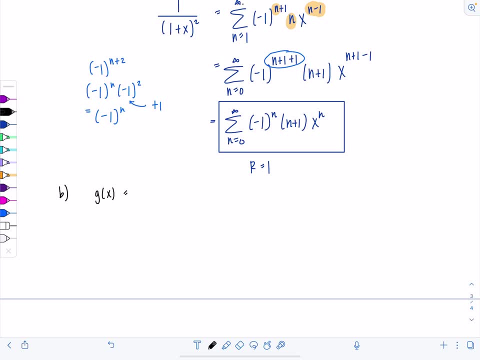 I want a power series for g of x equals 1 over 1 plus x. cubed. Ooh, Remember, this is already a power series. Let's erase this. This is already a power series for 1 over 1 plus x. squared right. 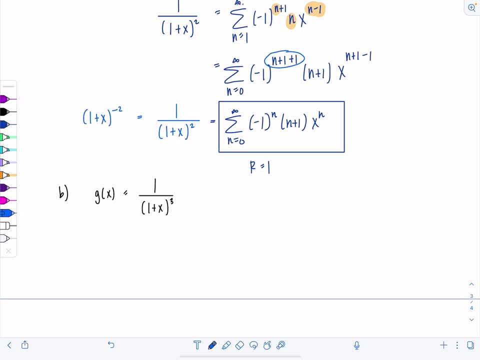 Which is 1 plus x to the negative second. So if I want to change the exponent in the denominator from 2 to 3, make it go up. take a derivative. So derivative With respect to x of 1 plus x to the negative second is going to be the derivative with respect to x. 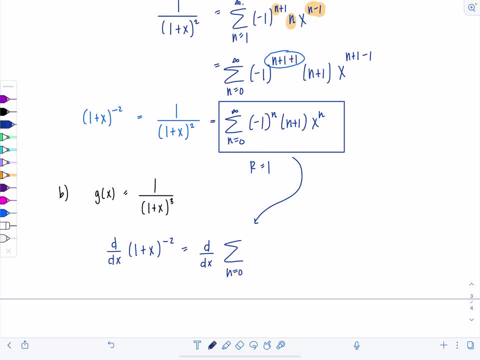 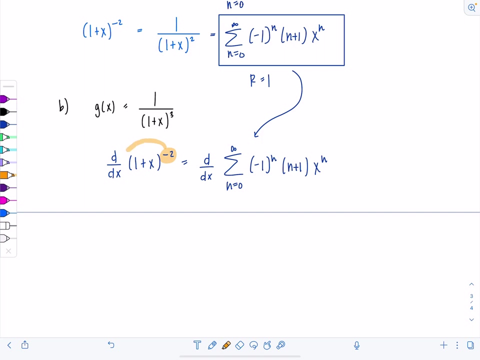 of this glorious power series we just found: n equals 0 to infinity. negative 1 to the n, n plus 1, x to the n. Okay, Let's see what emerges. So take the exponent, bring it down in the front. That's going to be negative 2.. 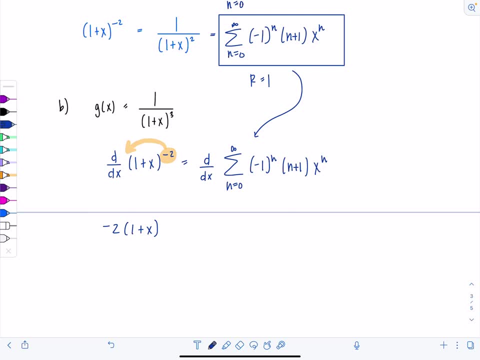 Leave that alone. Leave that alone. New exponent is going to be negative 3.. Good, And then derivative of the inside is just 1, so we don't need to do anything else. Now we're going to have the sum. Be careful. 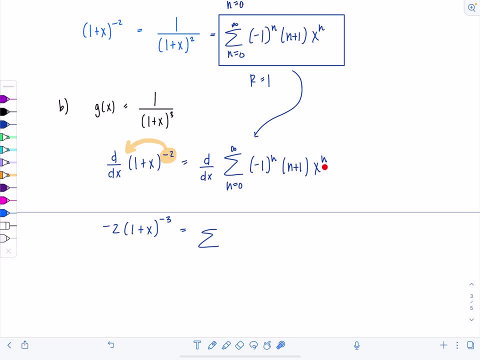 When n is 0, the first term is going to be a constant. So when I take the derivative it's going to go away. So the derivative needs to start at 1 to infinity. Don't have a meltdown. We're taking the derivative. with respect to x. 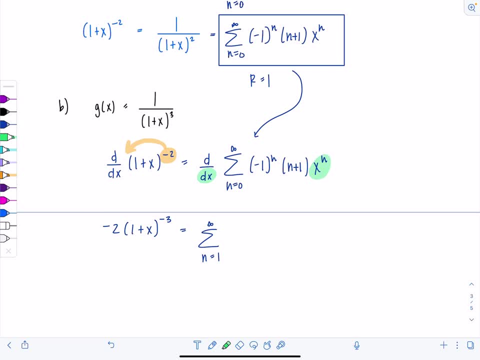 So everything besides x to the n is a constant, So it just comes along for the ride. Just rewrite it as is and then now take the derivative of x to the n. You can do that. You just did it a second ago. 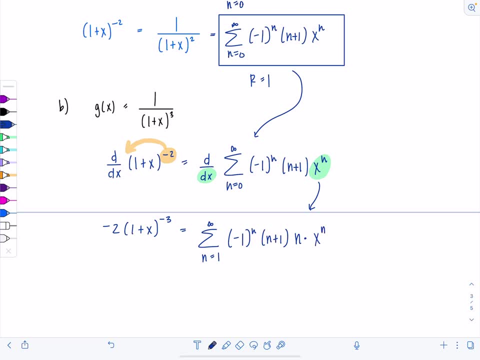 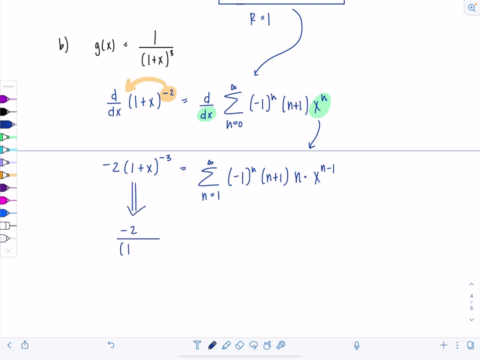 Bring the exponent down in front and then subtract. Now it's x to the n minus 1.. See, Look at us surviving, thriving, We're fine. Okay, Now look what's over here on the left-hand side: Negative: 2 over 1 plus x cubed. 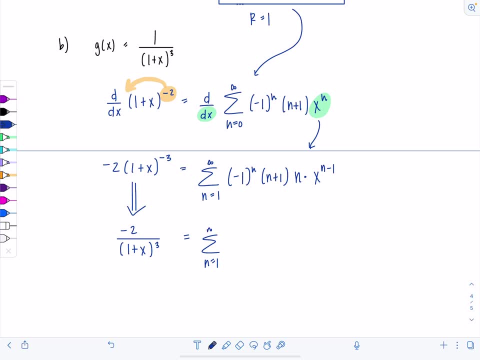 Okay, Is that what I want? Is that g of x? Not quite, Not quite people. What's there that I want to get rid of? Well, I'm looking at g of x. There's just a 1 in the numerator. 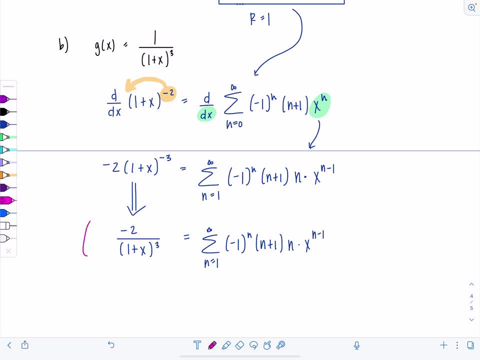 And here's a negative 2.. But we can get rid of it. We can just multiply both sides by negative 1 half. Hmm, Negative 1 half. I want to put it right there. Okay, So then this cancels. 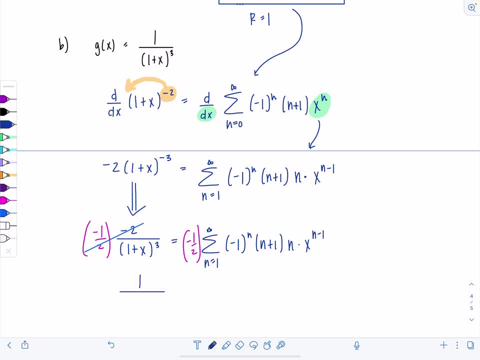 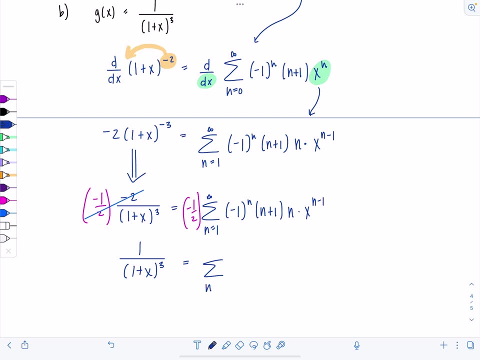 And then I have on the left-hand side 1 over 1 plus x cubed, And then this is going to be the sum n equals 1 to infinity. I'm going to leave the 1 half outside, But the negative I will incorporate with this negative 1 half. 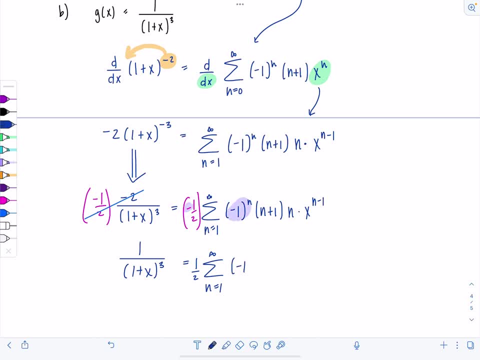 With this, negative 1 to the n. Okay, So then we'll have negative 1 to the n plus 1.. n plus 1.. And x to the n minus 1.. Okay, Lovely. No, Don't leave it like this. 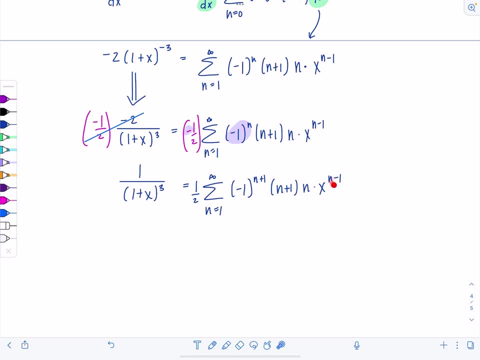 Because we want to try, if possible, to have our final answer. just have x to the n, So I want this to go up by 1.. So I'm going to replace all of the n's with n plus 1.. If I want that to go up, then I need to go the opposite direction. 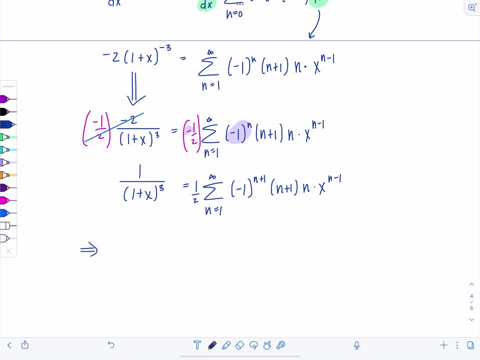 This needs to start at 0.. So we'll be done soon. 1 over 1 plus x cubed is Just leave the 1 half out there, right, There's no 2 inside to combine it with. Start at 0.. 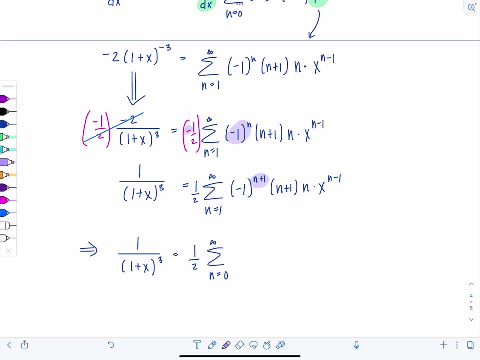 We talked about this. This is going to become negative 1 to the n plus 2.. But that's just the same as negative 1 to the n. This is going to become n plus 2.. This is going to become n plus 1.. 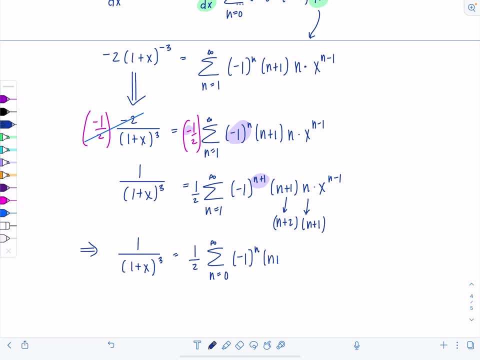 Okay, And then you'll have x to the n. Wow, wow, wow. Here's this one. What's the radius of convergence? Should we do a ratio test? Heavens, no, We found the radius of convergence of this guy. 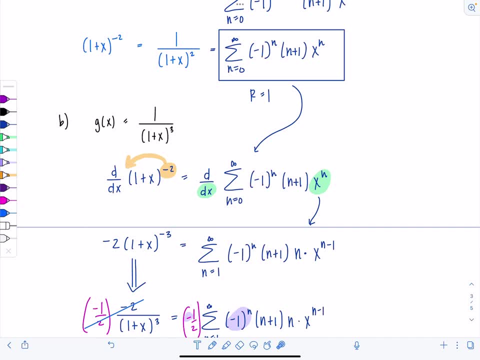 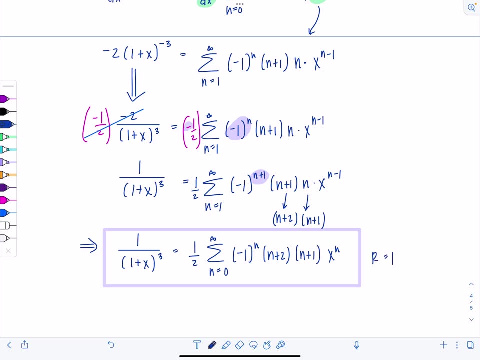 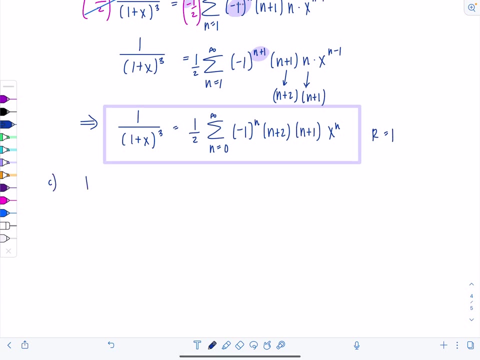 And it was 1.. And all I did was differentiate and just mess with some constants. So nothing's going to change, So it's still 1.. Okay, Last part to this problem. Example C: Say I wanted you to find power series representation for h of x. 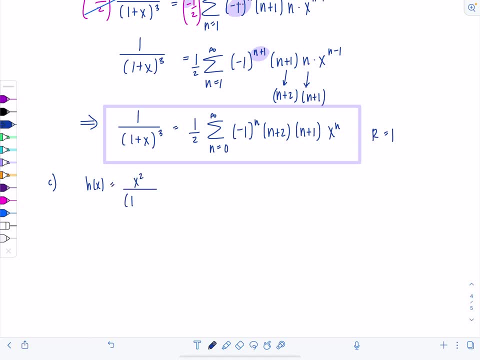 which is x squared over 1 plus x cubed. What would you do? Well, I already have a power series for 1 over 1 plus x cubed. The difference is I need an x squared now, So I should multiply this entire sum by x squared. 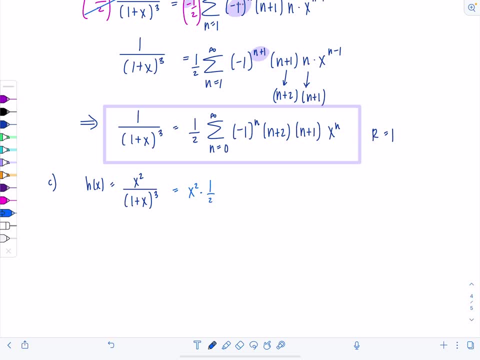 So that equals x squared times a half times the sum n. equals 0 to infinity, negative 1 to the n, n plus 2, n plus 1, x to the n. So I'm going to bring this and combine it with x to the n. 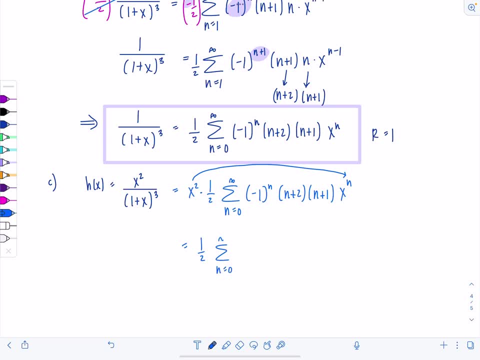 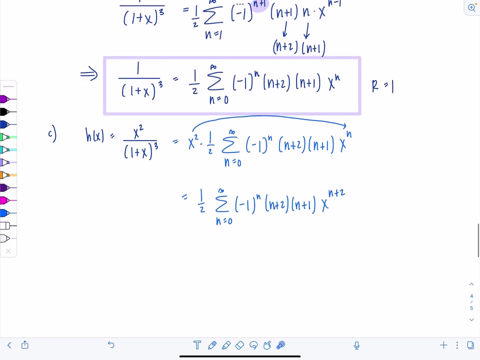 So then now we'll have: the sum n equals 0 to infinity negative, 1 to the n. n plus 2, n plus 1, x to the n plus 2.. Good, Should we adjust? Yes, I can write this as x to the power of n if I subtract 2 from all of the n's here. 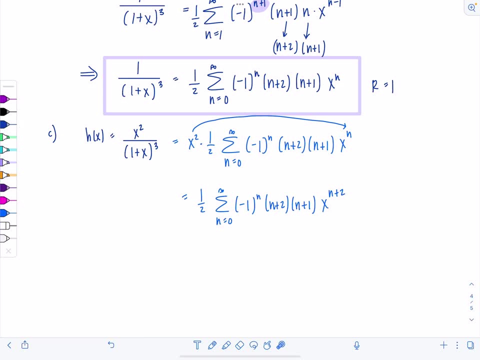 So if I want these to go down by 2, this needs to start 2 higher. So now I'm going to start at n equals 2.. I know kind of wild huh. And then negative 1 to the n minus 2 is also the same as negative 1 to the n. 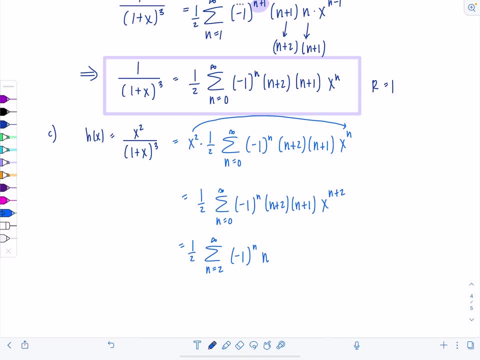 And then this is just going to become n plus 2 becomes n, n plus 1 becomes n minus 1, and then we have x to the n. Very lovely, Radius of convergence is still 1,. right, All I did was multiply by x squared. 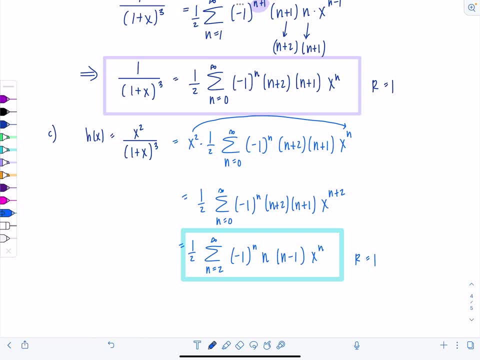 If you're too nervous, do a ratio test, Why not? Okay, So this is the second scenario. You have a higher power down there in the denominator, So you find a power series for the original, the original without the higher power. 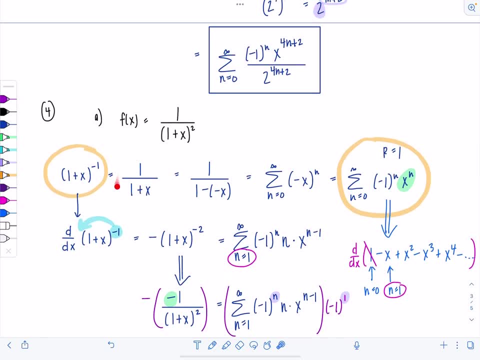 Remember how we started in the very beginning. just with 1 over 1 plus x, You get a power series and then you take the derivative. however many times you need to keep bumping up that exponent. All right, Last case. Last case is they give you? I want to see what number that was 4.. 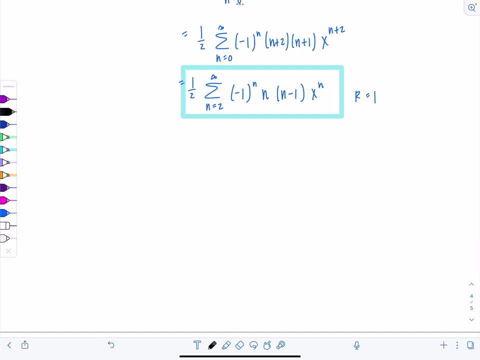 So last case is they give you some sort of function that has a natural log in it, Like why natural log? Because that's like the only other kind we can do. okay, We're running out of options, These are the only, and when you remind yourself of that, I think it makes it less intimidating. 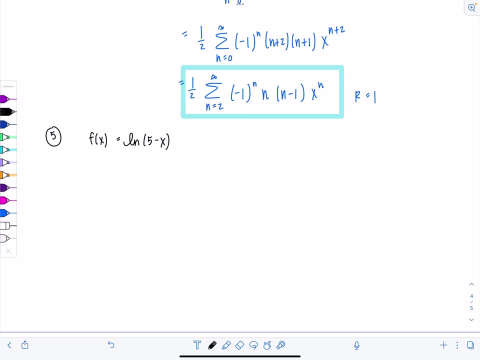 Like there's only three scenarios, you guys, So here's the third one: f of x is ln of 5 minus x. No Home base is 1 over 1 minus x, which is the sum. n equals 0 to infinity, x to the n. 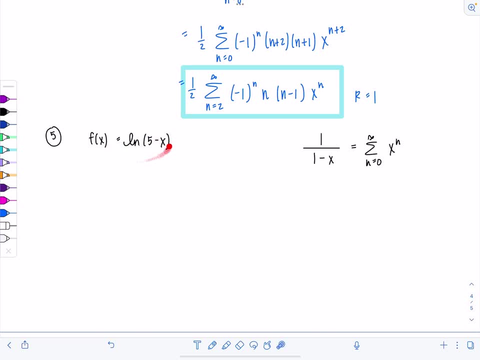 I cannot get a ln of 5 minus x to resemble this in any way right now. okay, What we do is we take the derivative Always f, prime of x. So derivative of ln, something is 1 over the something And then by the chain rule you have to multiply by the derivative of the something of what's inside. 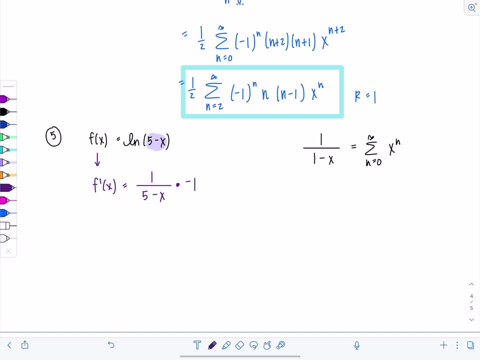 So derivative of 5 minus x is negative 1.. So let's see This is negative 1.. I'm going to put that in the front Over. I'm going to factor out a 5 times 1 over 1 minus x over 5, right. 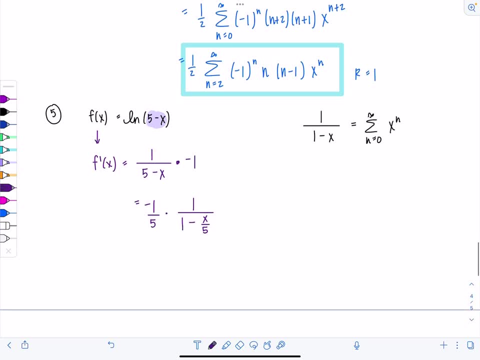 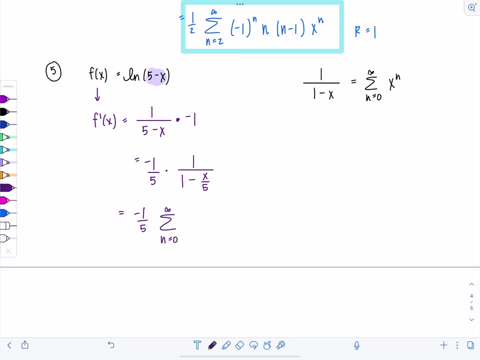 Can we get a power series for this bad boy? Certainly So. we have negative 1.. So we have negative 1 fifth times. the sum n equals 0 to infinity x over 5 to the n. If you want radius of convergence right now, let's do it. 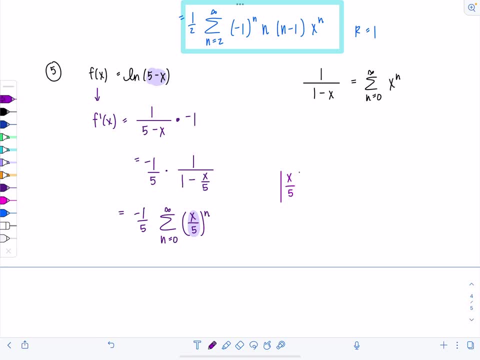 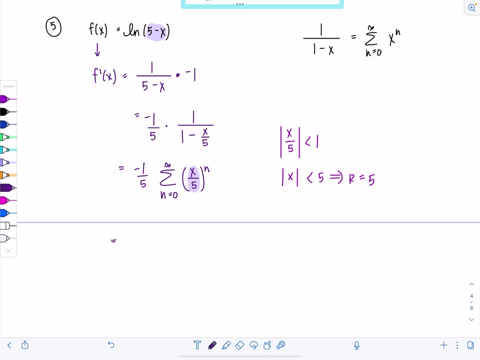 So we require absolute value of x over 5 to be less than 1, which means absolute value of x is less than 5.. So radius is 5,. okay, Can we simplify this sum further? Yes, I'm going to bring in. leave the negative out, because you see how it's. there's no negative in here being raised to the n. 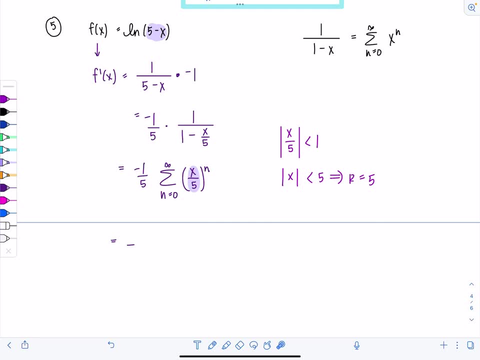 It's not alternating, It's just like one lonely negative. He can stay outside. And then we have the sum n equals 0 to infinity, x to the n over 5 to the n plus 1.. Now remind yourself: who does this power series represent? 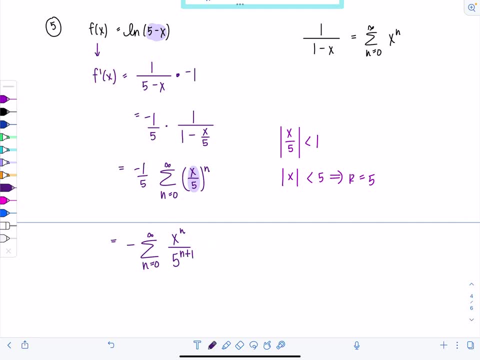 F, prime of x. Oh, okay, So we didn't quite do what we were asked. We found a power series, but not for the original function, for its derivative. How do I get back to the original function if I have its derivative? 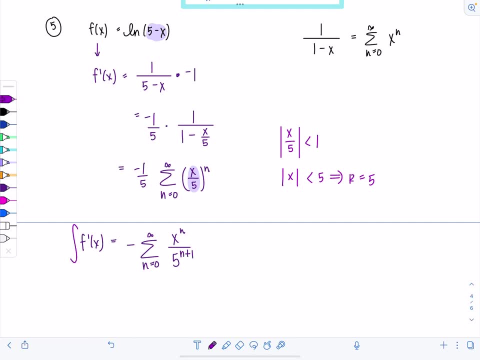 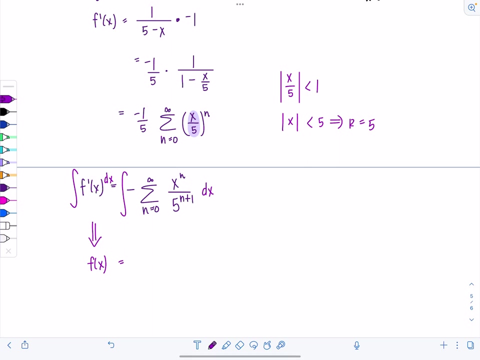 Well, you take an antiderivative right, Also known as an integral, thanks to the fundamental theorem of calculus. Ba-boom, Ba-boom. Please don't forget your dx, It makes me angry. Okay. So then now over here, we've got f of x equals. don't be scared to integrate an infinite series. 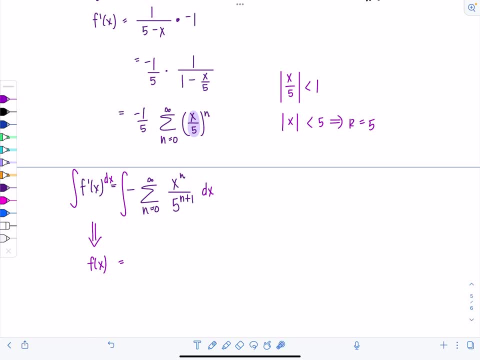 Okay, I know It can be overwhelming, but just remind yourself this: and this are just constants, because I'm integrating with respect to x, So focus on where x is, because nothing else is changing. Okay, In fact, just rewrite it right now so you stop stressing. 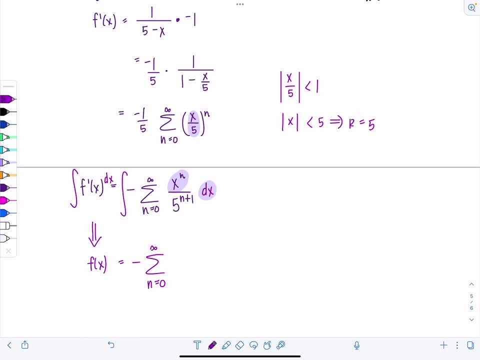 This negative. keep that there n equals 0 to infinity. When you integrate you add 1 to the exponent, So it's going to be x to the n plus 1.. And then you divide by the new exponent And then I still have that 5 to the n plus 1 down there. 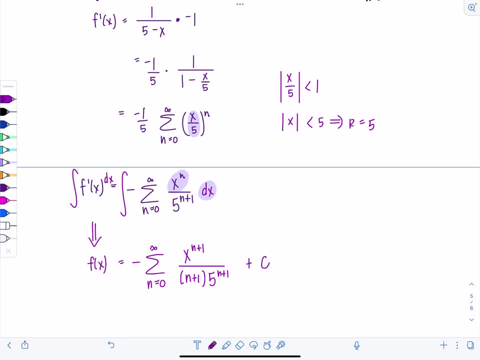 Plus c. Yeah, That's it literally. Okay. How can I find c? Well, look at where the power series is centered. It's centered at 0.. How do I know that? If it wasn't centered at 0, it would look like this: 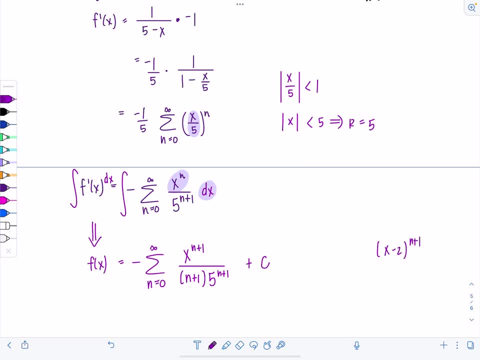 It would look like x minus 2 to the n plus 1, or something like that. You know what I mean Over blah, blah, blah. That's when it's centered at x equals 2.. So then you would plug in 2 for x. 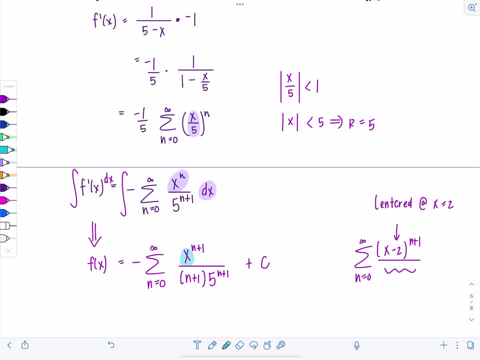 You want to plug in whatever value of x will make every single term in this sum 0. That way it goes away and you can solve for c. Okay, So in this case that number is 0.. Most of the time it is 0, you guys. 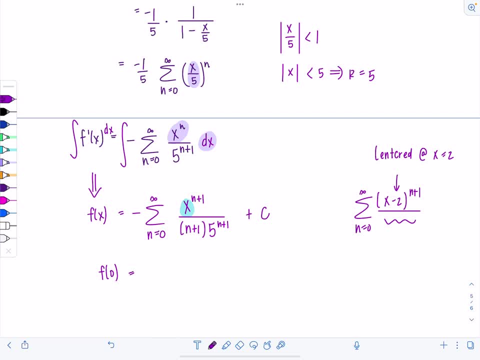 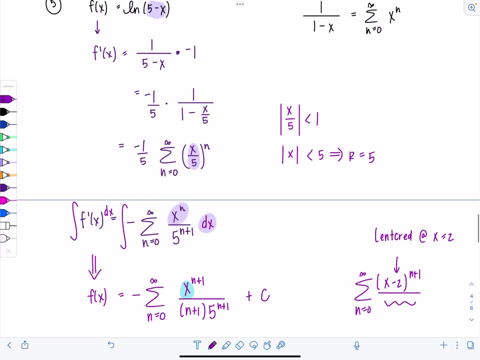 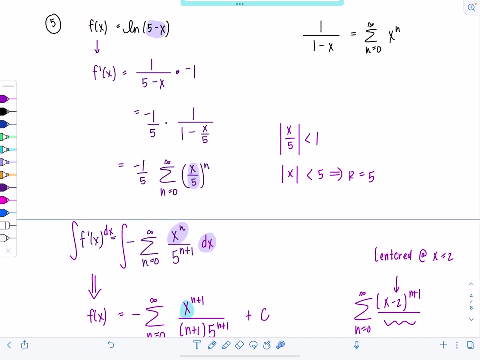 Okay, So f of 0 equals the sum of 0 plus c. And how does this help me find c? Well, I have f of x right here. f of x is ln of 5 minus x, So f of 0 is ln of 5.. 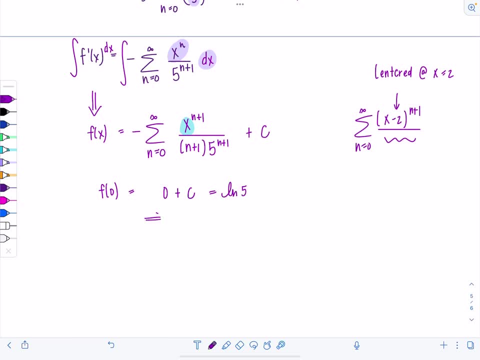 So that tells me c equals ln of 5.. So then now I can write: f of x is negative. sum n equals 0 to infinity, x to the n plus 1 over n plus 1, 5 to the n plus 1 plus natural log of 5.. 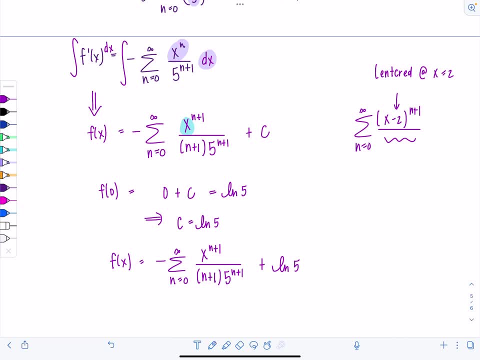 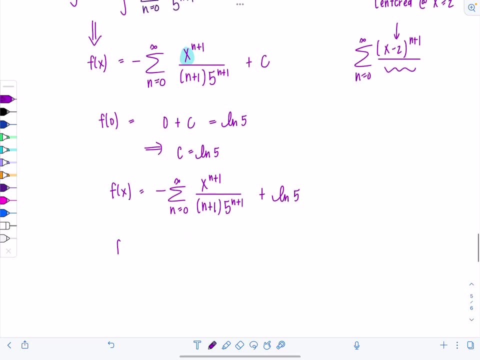 Can we clean up? We certainly should. I can write this as x to the n if I start at 1.. Okay, So let's do that. So then f of x is. it would look better. Let's put the ln of 5 first and then the minus sign. 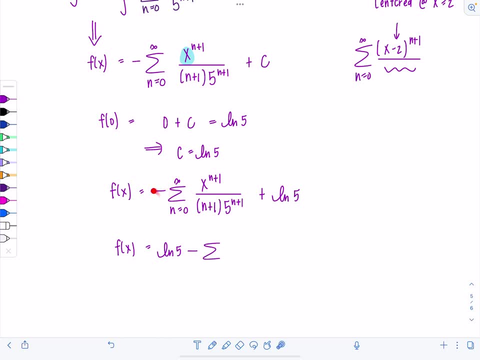 Like: hopefully at this point you have some aesthetic appreciation right. That like starting with the negative is not cute. n equals 1 to infinity. And then we have x to the n over n times 5 to the n. Radius of convergence is 5.. 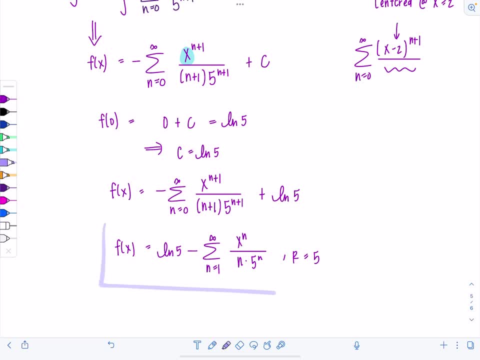 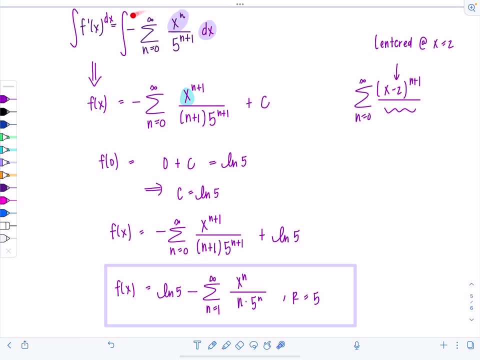 Wow, Do you feel fancy? I asked my class the other day. I'm like: did you ever think you'd be integrating an infinite sum? Be proud of yourself, Look at where you are. Okay, So that's the third scenario. 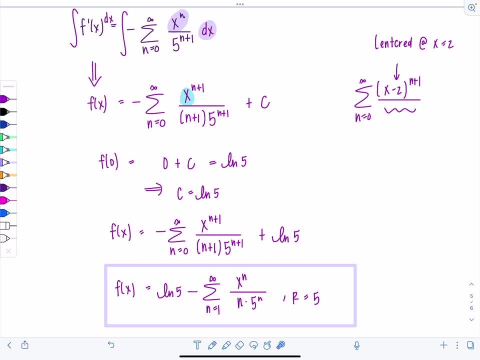 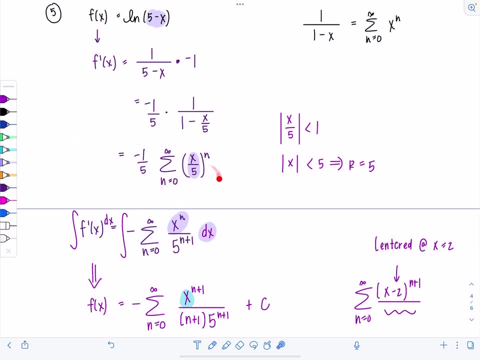 You have ln and you're like whoa. So I'm going to take the derivative first, Find a power series for the derivative and then integrate that power series so you can get the derivative, So you can have a power series for the original. 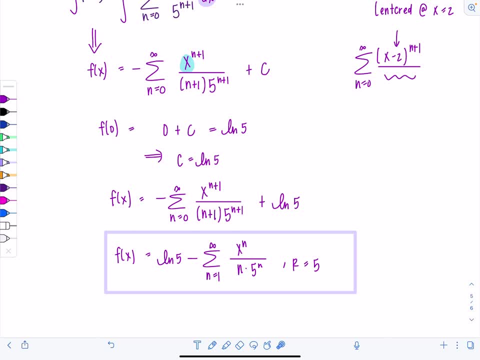 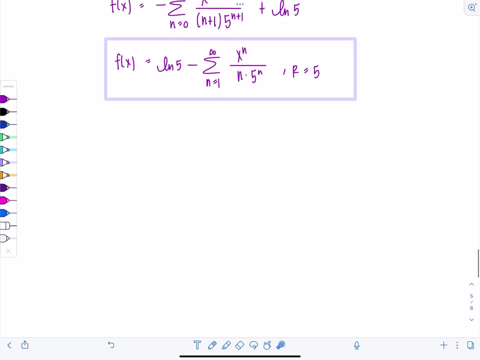 Okay, Great. So from here, what I'm going to do is a couple from the practice exam, So my students can be excited. Here we go, Same directions. I think this is number six. Again, f of x is 1 over 1 minus 6x squared. 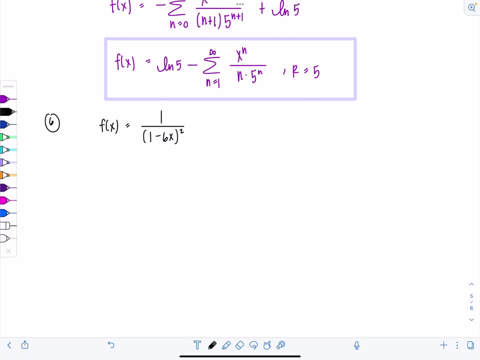 Okay, Which scenario is this? Can I just manipulate algebraically multiplying and dividing? No, Since I have this exponent here, what I'm going to have to do is first start with a power series for 1 over 1 minus 6x. 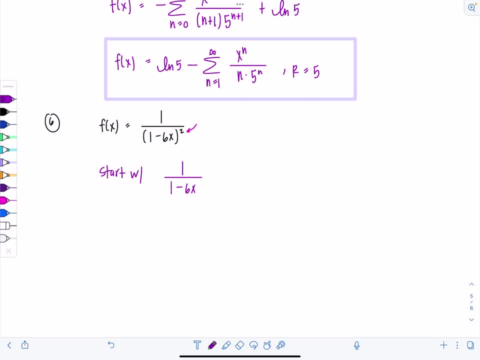 And then I'll take its derivative To bump up that exponent. So power series for 1 over 1 minus 6x is going to be: the sum n equals 0 to infinity, 6x to the n. So 1 over 1 minus 6x is the sum n equals 0 to infinity, 6 to the n, x to the n. 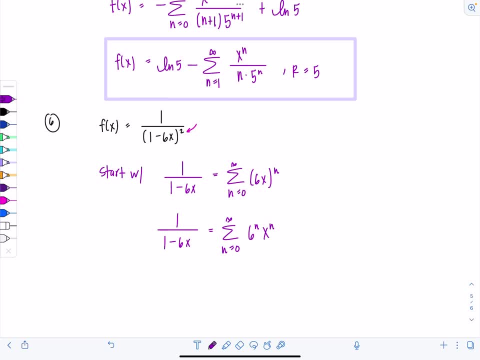 All right, Great, Is that what we want, though? Now I need the denominator to be 1 power higher, So I'm going to take a derivative. I'm going to rewrite this, though, as 1 minus 6x to the negative first. 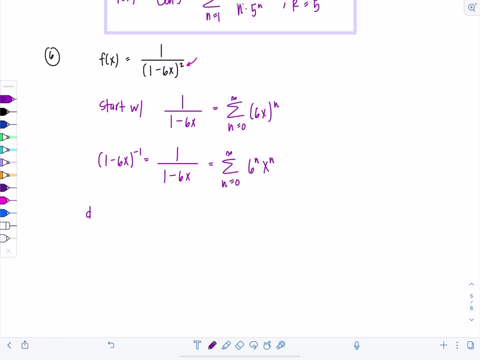 Okay, So the derivative with respect to x of 1 minus 6x to the negative first. So bring the exponent down in front, Subtract 1.. And then this time, when we do the chain rule, what's the derivative of the inside? 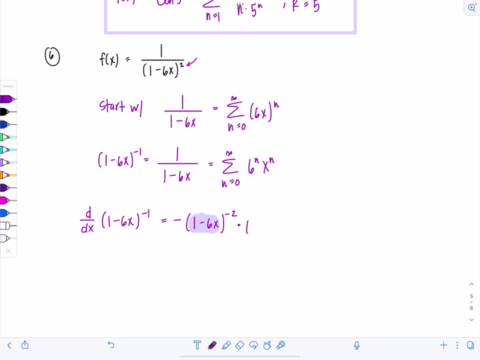 It's negative 6.. Very good, This equals the sum. Now be careful: The first term when n is 0 is a constant. So when I take the derivative it's going to go away. So n has to now start at 1 to infinity. 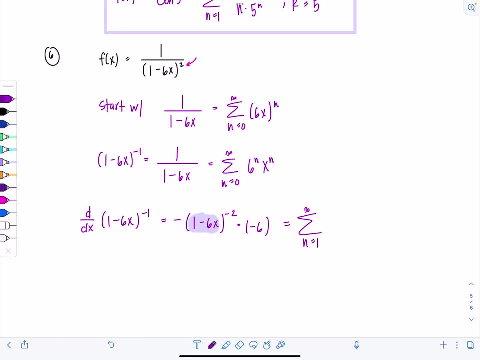 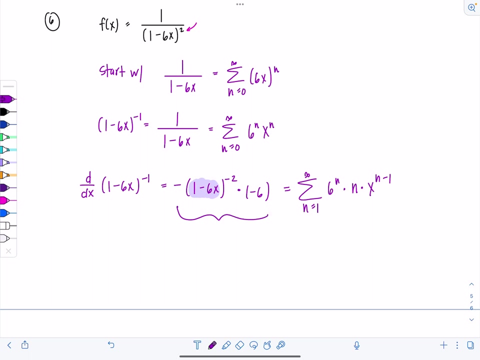 Only x is my variable, So 6 to the n just hangs out. When I take the derivative of x to the n, it's n times x, n, it's n times x to the n minus 1.. Okay, okay, So let's see what is this If I clean it up. 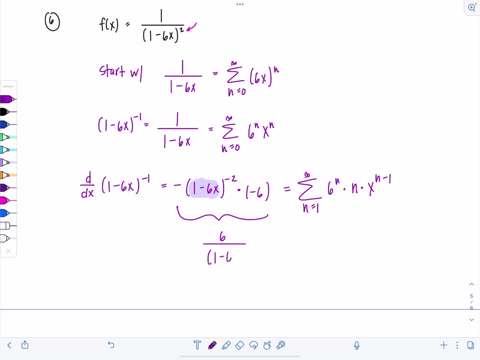 it's positive 6 over 1 minus 6x. squared, this is the sum. n equals 1 to infinity, 6 to the n, n, x to the n minus 1.. Is that my f of x? Is that u f of x? No, not quite. Look at this. 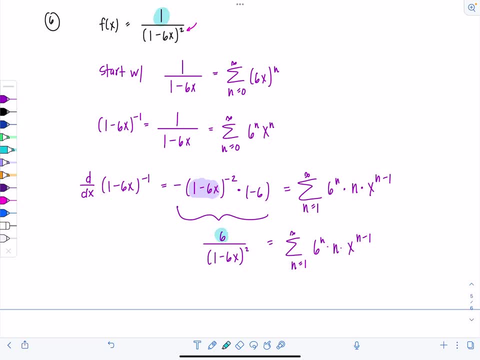 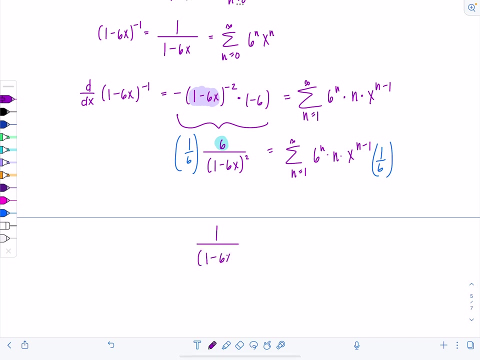 6, it need not be there. So how do we get rid of it? Very good, multiply by 1 sixth, 1 sixth. So then now, woohoo, we have 1 over 1 minus 6x squared, and this equals the sum. 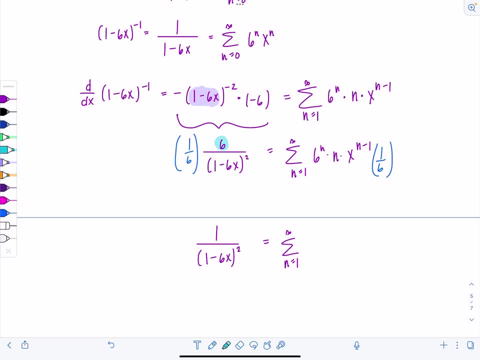 n equals 1 to infinity. Watch this: I have 6 to the n divided by 6 to the first, so I have 1 over 1 minus 6x squared, and this equals the sum. n equals 1 to infinity. 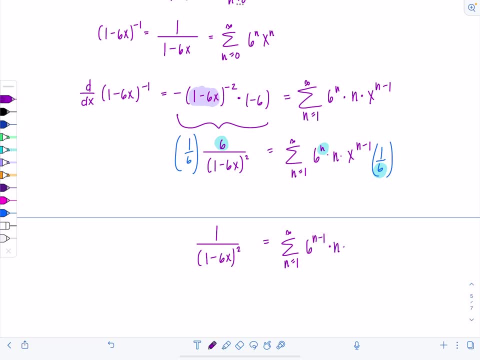 So now I have 6 to the n divided by 6 to the first, so I have 1 over 1 minus 6x squared, so that's going to be 6 to the n minus 1 times n times x to the n minus 1.. 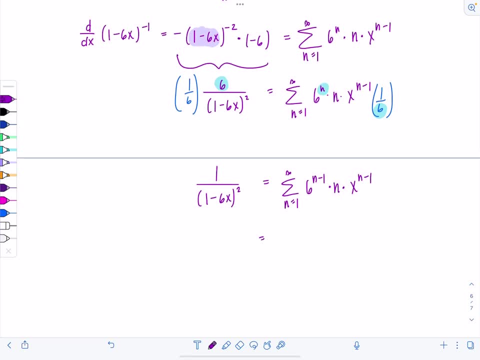 And no, we don't want to leave it like that. I want x to be raised to the n. So if I want this to start at n and I want to add 1 there, I got to start 1 lower, So we'll. 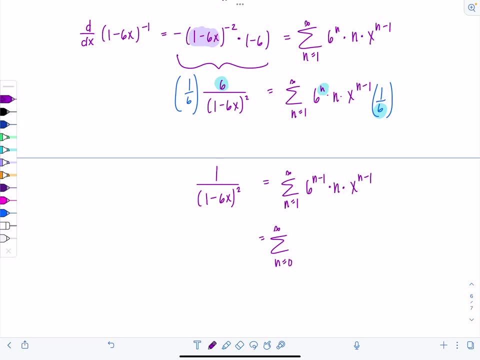 start at n equals 0 to infinity, and then we'll have 6 to the n times n plus 1 times x to the n, And that just looks weird to me. so I'm going to put the n plus 1 first, Isn't it looking ugly? 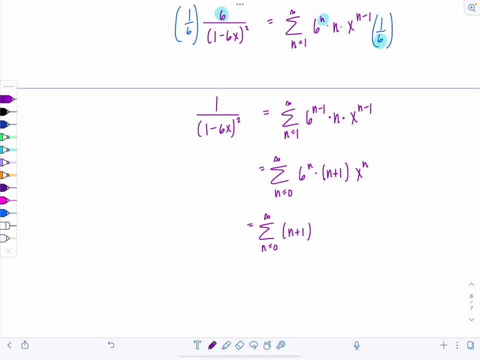 Oh no, n plus 1, 6 to the. that's better, yes, And then I'll just say this equals f of x. Okay, beautiful, beautiful, beautiful, Okay. I got another one for you. This time it's going to: 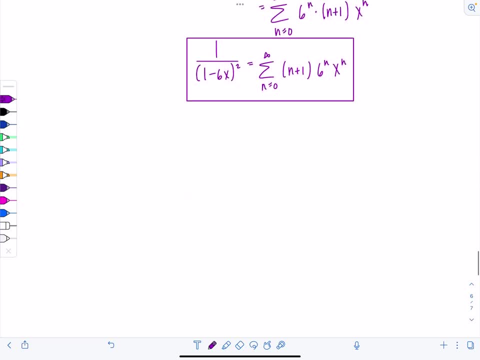 involve ln. I don't even know what number I'm on, Okay, I think 7.. f of x equals x squared ln. 1 plus 4x. Ooh, okay, Don't worry about this. x squared till the bitter end, the bitter end, okay. 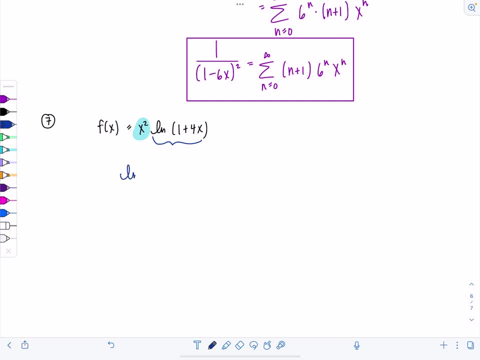 First. we're just going to start with ln 1 plus 4x. Can you find a? Do we have a power series for this? No, We take the derivative first and then we'll find a power series for it. So the derivative of ln of 1 plus 4x is 1 over 1 plus 4x times. don't forget the. 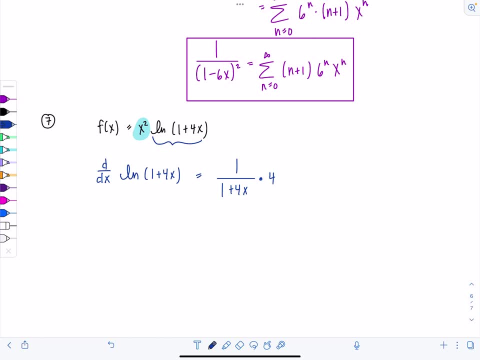 chain rule times 4.. Okay, so that's let's see 4 times 1 over 1 minus negative 4x. right, You see where this is going Good, So this is going to be 4 times the sum n equals 0 to infinity. 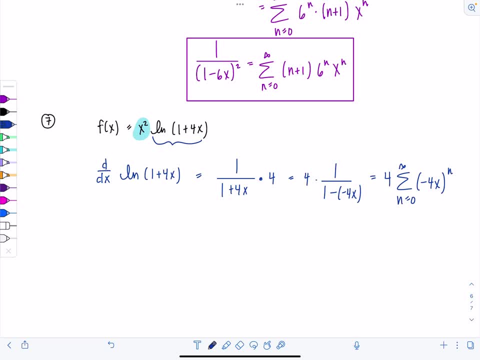 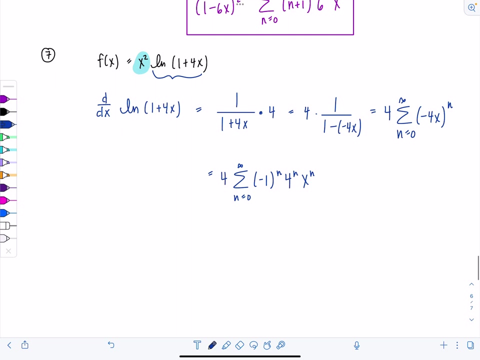 negative, 4x to the n. Let's clean it up. So that's 4 times the sum. n equals 0 to infinity negative, 1 to the n, 4 to the n, x to the n. And then, look, we should combine these 4s right. 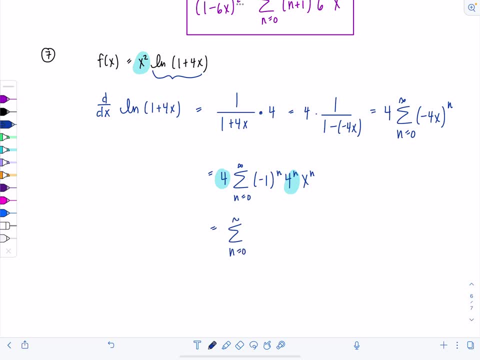 Okay, so then that's: the sum n equals 0 to infinity negative, 1 to the n, 4 to the n plus 1, x to the n, And this is the derivative of ln of 1 plus 4x. Well, how do I get back to ln of 1 plus? 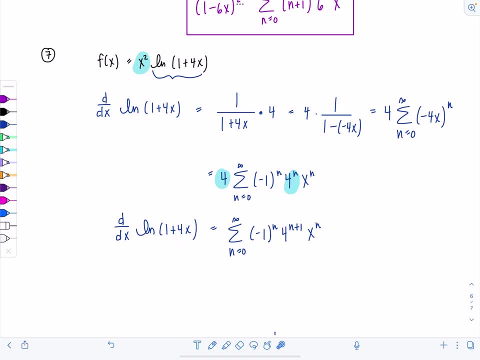 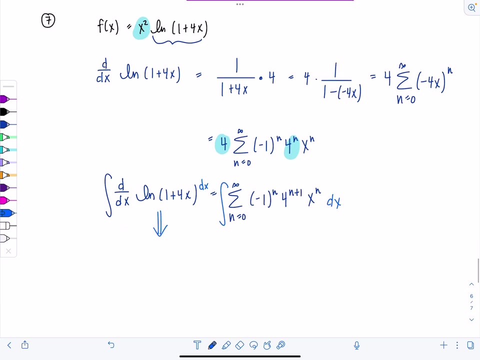 4x. This is a power series for its derivative To undo a derivative we have to integrate. So then now if I integrate the derivative, I just get back ln 1 plus 4x. And then here's where I have to always just give you a little pep talk. I know there's a lot of scary stuff. 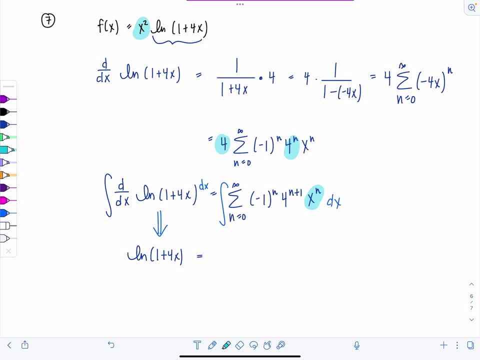 going on, but this is the only x in that integral, So everything else just stays the same. It doesn't change, It's just a constant. n equals 0 to infinity. negative 1 to the n, 4 to the n, x to the n. 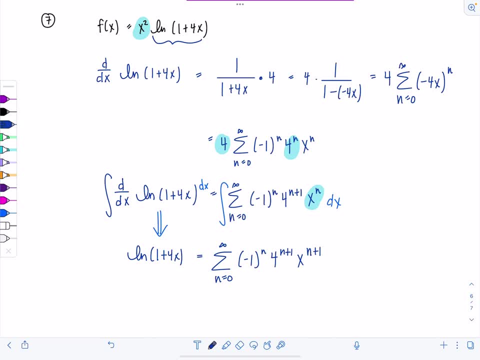 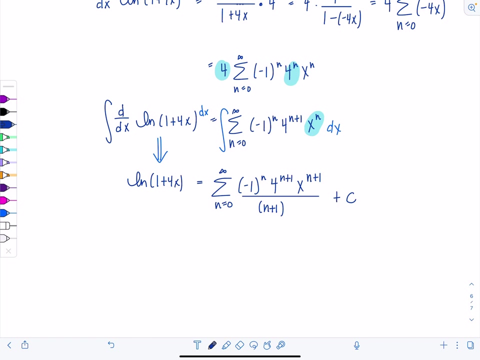 4 to the n plus 1, add 1 to the exponent, divide by the new exponent and we pick up a plus c. Good See, Okay, now from here we have to find c. So where is this power series centered at 0?? 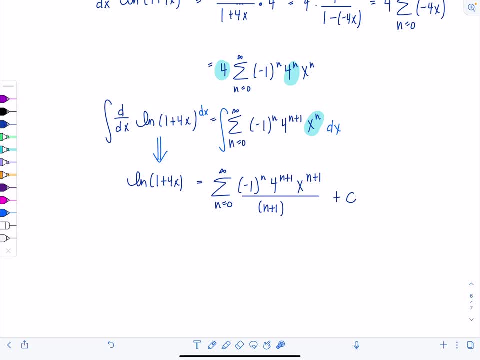 Remember, if it's not centered at 0, it would be like x minus or x plus some number in parentheses. I don't see that. I'm going to plug in 0. So I have ln of 1 plus 0 equals the sum of a bunch of 0s plus c. 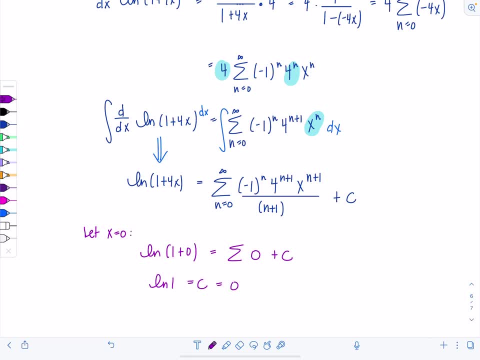 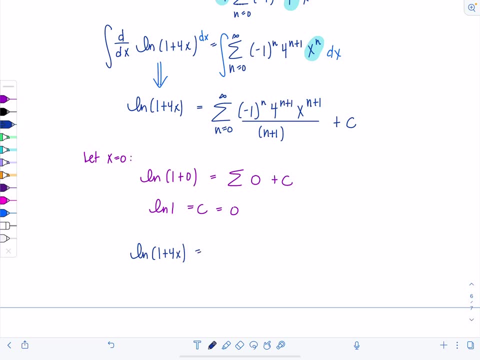 So ln of 1 equals c, which is 0.. Okay, So that means now I have: ln of 1 plus 4x equals the sum, n equals 0 to infinity negative, 1 to the n, the n plus 1, x to the n plus 1 over n plus 1.. Okay, good, Good, good, good. Is that what we? 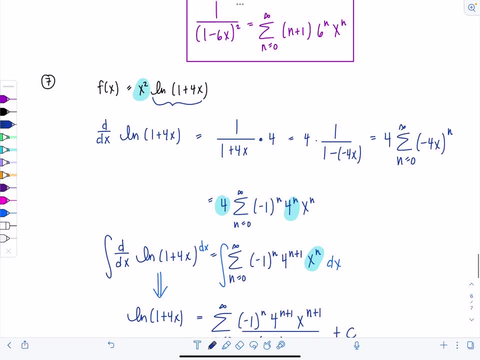 wanted, though Not quite. I have a power series for ln of 1 plus 4x. What's missing? x squared. I told you, save it for the bitter end. This is the bitter end, So I'm just going to go ahead and 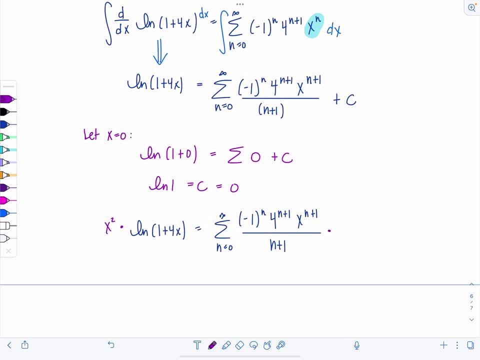 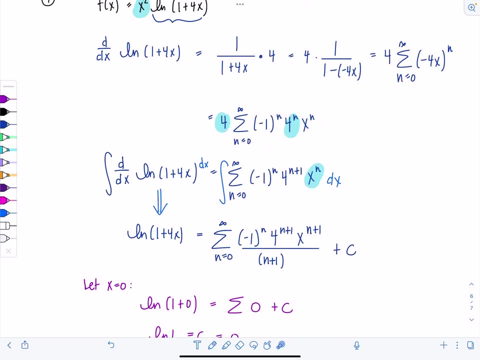 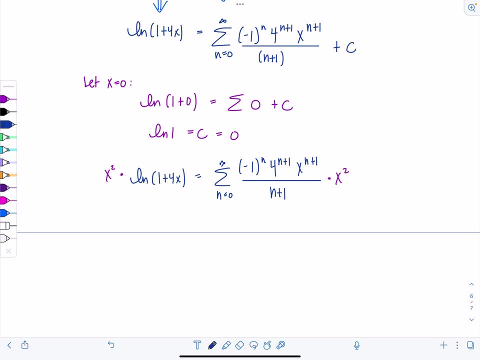 multiply both sides now by the x squared. Okay, and one mistake I saw a lot of my students do yesterday. they wanted to put it in too early. I think it just makes it more confusing. Okay, I would wait until the very, very end to just multiply by extra stuff. So then we have x. 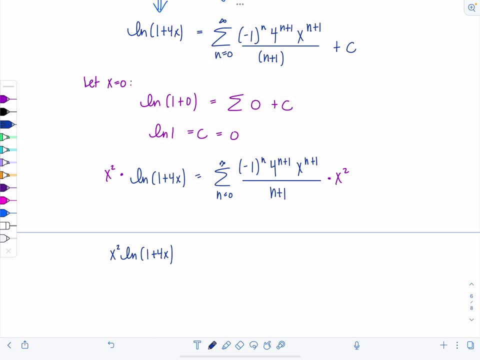 squared ln. 1 plus 4x equals the sum. n equals 0 to infinity, negative, 1 to the n, 4 to the n plus 1, x to the n plus 3, now over n plus 1.. Okay, do we want to lower this by 3 and start this at 3?? 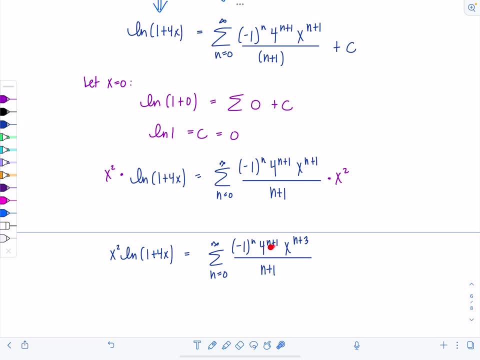 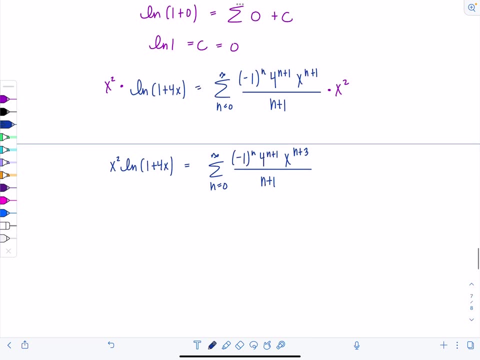 This would then become n minus 2.. I don't think so. I would say let's just start at n equals 1, and then this is a kind of rare case where it probably doesn't look better To have xb to the n. So now I'll have negative 1 to the n minus 1,. 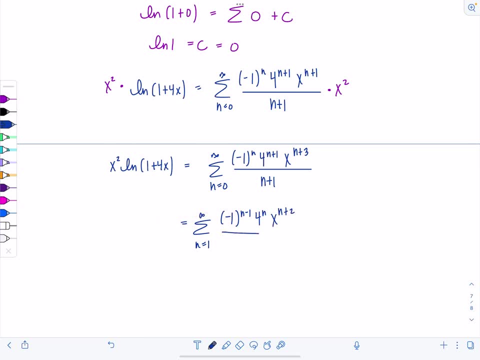 4 to the n, x to the n plus 2 over n. So what did I just do? I started the index one higher. so then I have to subtract 1 from all of the expressions involving n here. I think that's the cleanest way to write it. Let me show you: If we were to try to have xb to the n, 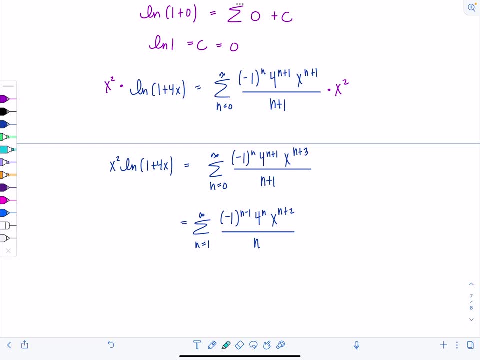 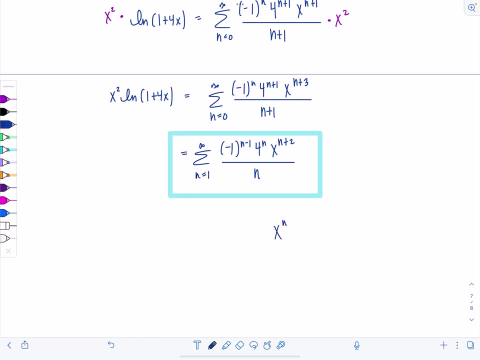 then I would need to Excuse me. Maybe this is not Okay. If you wanted to start at x to the n, then you would need to start the sum at: n equals 3, and then you would subtract another 2.. 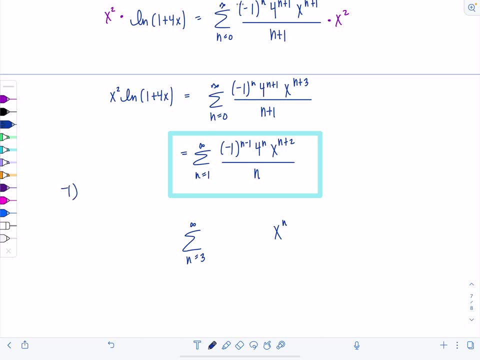 So I would have negative 1 to the n minus 1 minus 2, which is n minus 3.. That's negative 1 to the n times negative 1 to the negative third. That's negative 1 to the n. This is still just negative 1, right. 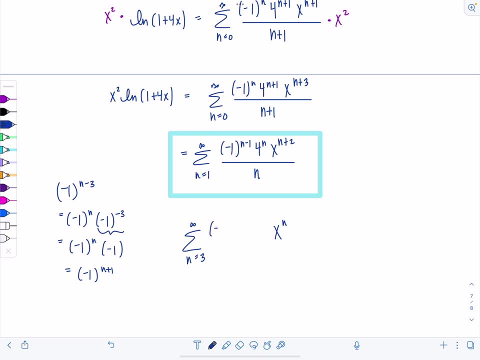 So you could write it as negative: 1 to the n plus 1 or n minus 1.. It doesn't matter. Then 4 would be to the n minus 2, and then the denominator would be n minus 2.. I don't think that looks better, you know. 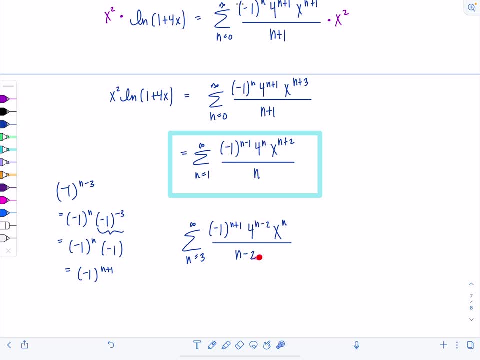 This matching looks better than having this extra chaos. So I would say, just stop here. This is like a rare case where it's better to just leave it as n plus 2. But check with your professor. Whatever they want, make them happy, Literally. 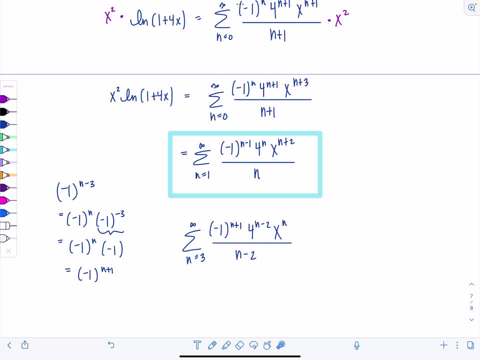 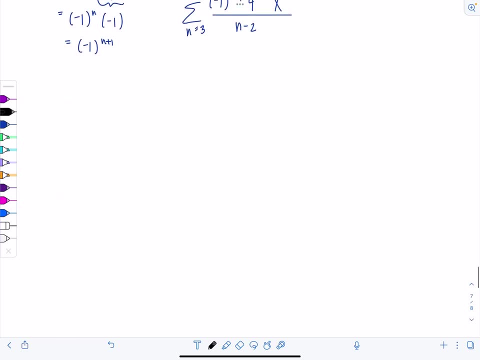 Okay, Last one. It's a fun spicy one. Okay, Yes, I think I called that one 7, so I'm calling this one 8.. Um, where did it go? Here it is f of x. is ln 1 plus x cubed over 1 minus x cubed. 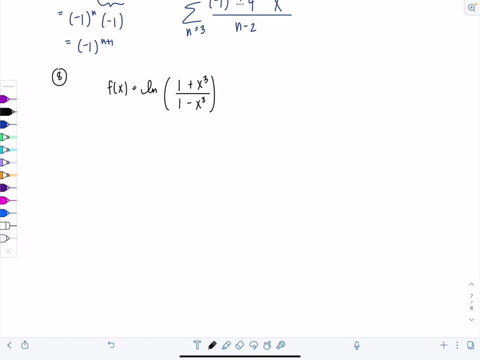 Okay. So when you see ln, you go, ooh, I'm not going to try to find a power series with this guy, I'm going to take the derivative first And I'm not going to just jump right in and take the derivative right now because I would have to do such ugly chain rule right involving the quotient rule. 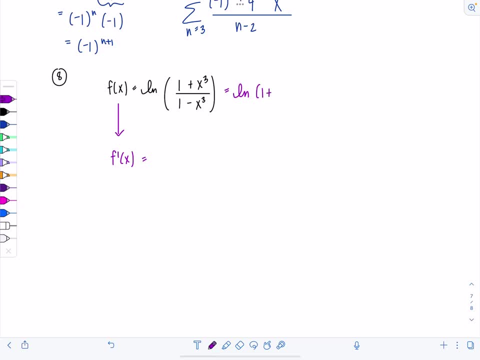 So I'm going to use my log properties and write this as ln 1 plus x cubed minus ln 1 minus x cubed. So now let's take the derivative. So derivative of ln of something is 1 over the something times the derivative of whatever the something is. 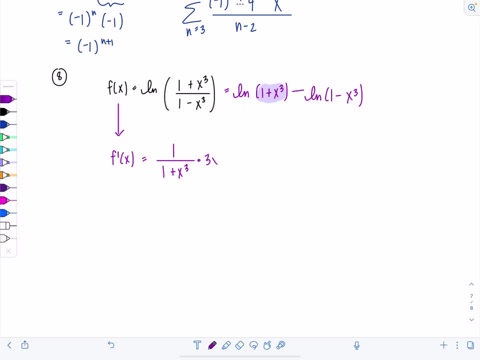 In this case, derivative of Of 1 plus x cubed is 3x squared Minus. the derivative of the other term is going to be similar: 1 over 1 minus x cubed times negative 3x squared right. 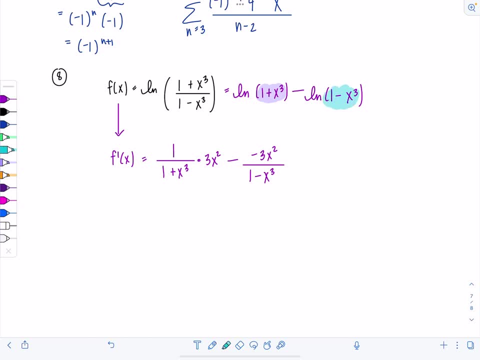 That's the derivative of the inside. here There's its derivative. So what does this turn into? This turns into 3x squared over 1 plus x cubed, Plus 3x squared over 1 minus x cubed, And this is f prime of x. 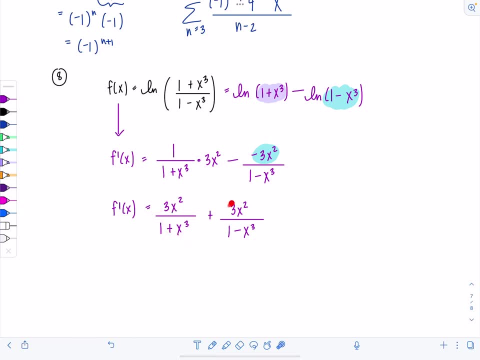 Now you could try and get a power series for each of them right now, and then there is a way to combine them into one sum. It's just a little more work. What's easier is to combine them right now, And this is a special kind of case where it works out nicely because you see how the denominators are conjugates. 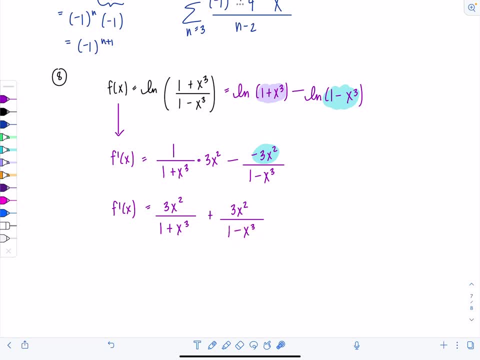 It's going to turn out so pretty Watch. So I'm going to clean up and get a common denominator. So I'll multiply this guy by 1 minus x cubed top and bottom, and then this guy by 1 plus x cubed. 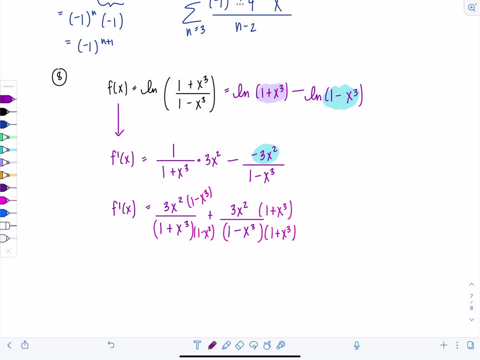 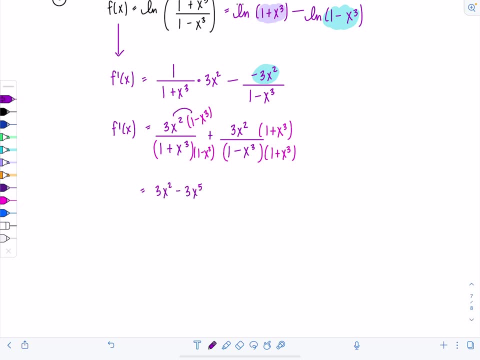 All right. So now we have 3x squared minus 3x to the fifth. I'm just distributing Plus 3x squared plus 3x to the fifth Over 1 plus x cubed times 1 minus x cubed. 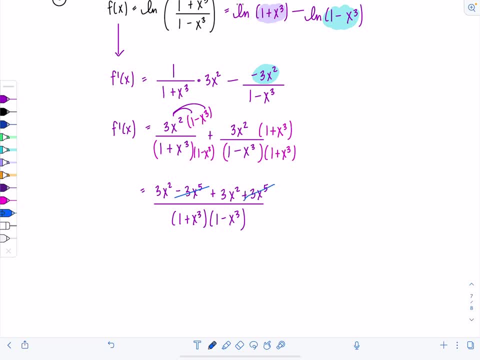 And the cool part is see how these 3x to the fifths just cancel Good. So then f prime of x is 6x squared over. if I multiply out the denominator, what do I get? It's 1 minus x to the sixth. 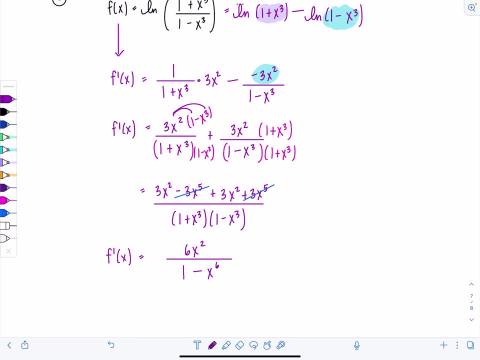 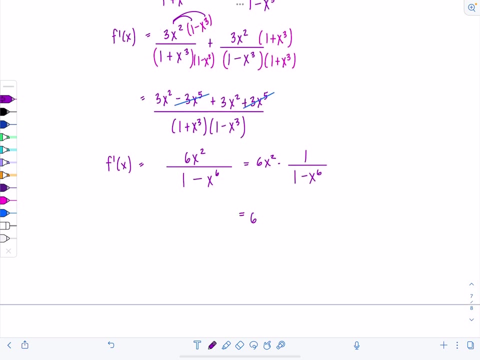 You can find a power series for this really easy, Can't you? Yeah, it's just 6x squared times 1 over 1, minus x to the sixth. So then that's 6x squared times, the sum n equals 0 to infinity, x to the sixth. to the n. 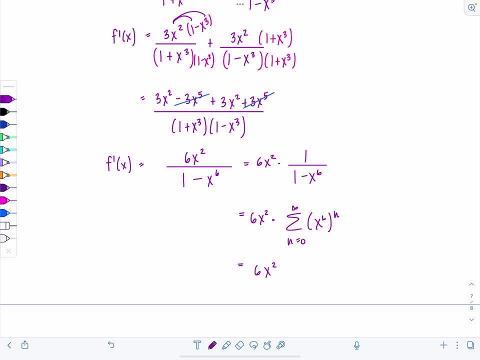 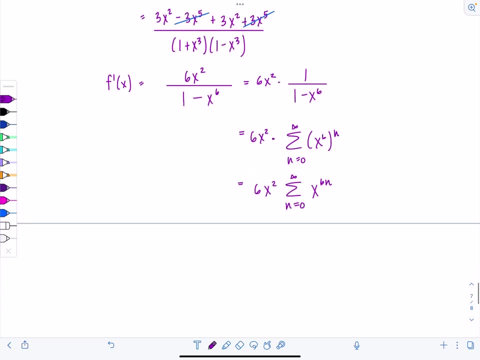 Oh, And then this is 6x squared times the sum n equals zero to infinity, x to the 6n. And then we're almost done. This is 6 times the sum n equals zero to infinity x to the. I want you to combine these right now: 6n plus 2, right. 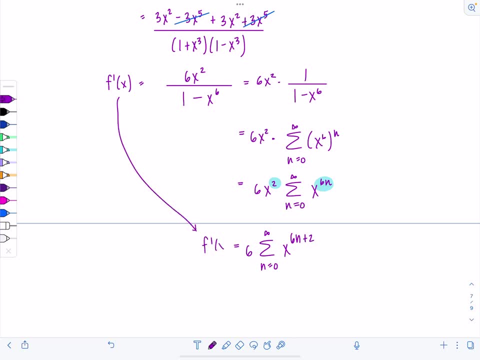 Good, And this is all the power series for f prime of x. Yes, Good, The worst is over, I promise. So now, how would I find a power series for f of x? I have one for f prime. How do I go backwards? Integrate, Integrate, Okay. 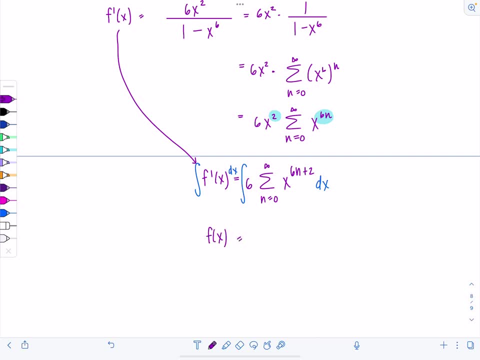 So then, f of x equals no panic attacks. just add one to the exponent. divide by the new exponent, leave everything else alone. Leave it alone 6 times the sum n equals zero to infinity. Add one, it's going to be x to the 6n plus 3, divided by 6n plus 3, plus c- Yeah, don't forget the plus c. 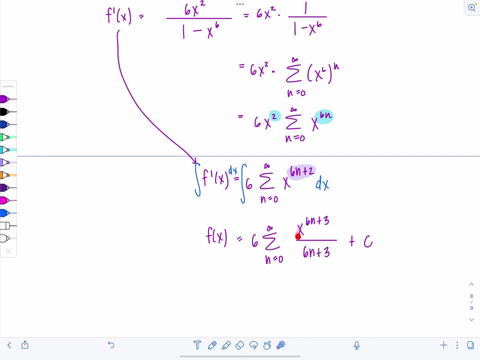 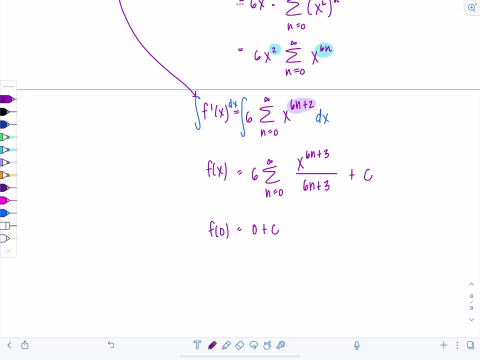 We're going to solve for it really quickly. This guy's centered at zero, so I'm just going to plug in zero for x. So f of zero equals zero, Zero plus c. Do you remember what f of x was the original? It was ln 1 plus x cubed. 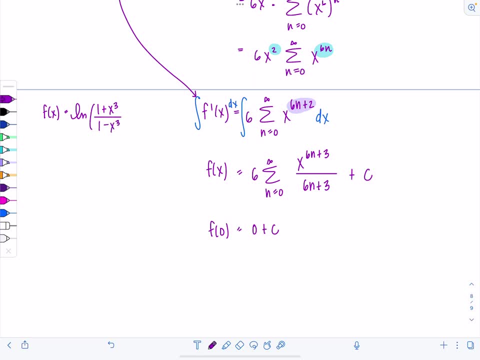 over 1 minus x cubed. So f of zero is ln 1 plus 0 over 1 minus 0, which is ln of 1. So that's zero. So c is zero. How boring, I'm sorry, Okay. 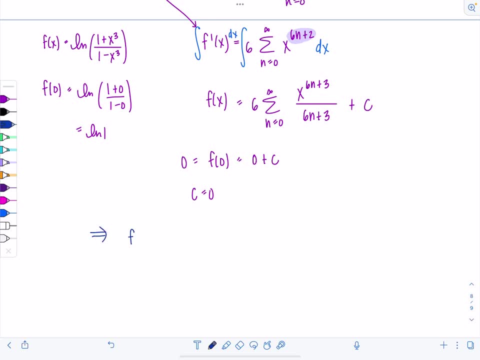 Now we can put it all together. So f of x is 6 times the sum. n equals zero to infinity, x to the 6n plus 3, over, you know, I can factor out a 3 from here, And then I have 2n plus 1,.